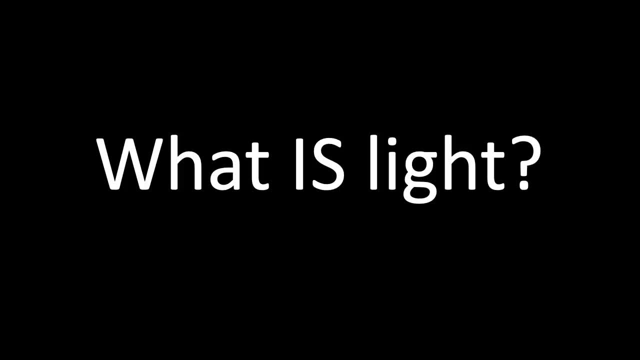 To answer this question would require thousands of years of experimentation and theoretical inquiry, and would involve a selection of the most famous scientists of all time, weaving together ideas across generations, overthrowing long-held ideas of the past and the present and the future. 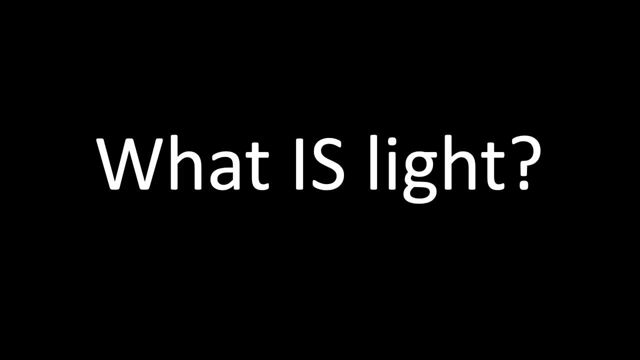 Ideas and beliefs and forever changing the way that we view the universe. So what is light? To even pose this question represented a huge leap forward in our attempt to understand the universe, to believe that light is some thing that can be investigated. But if light is a thing, then what kind of thing is it? Some of the earliest documented theories: 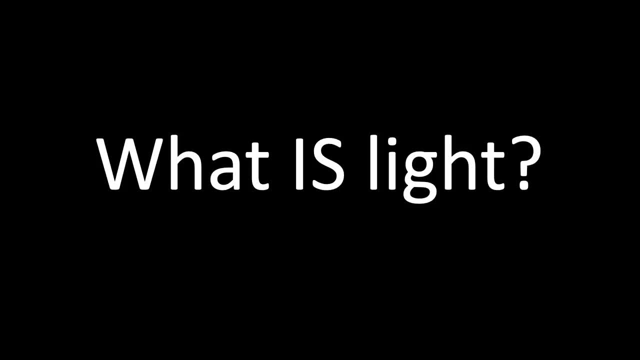 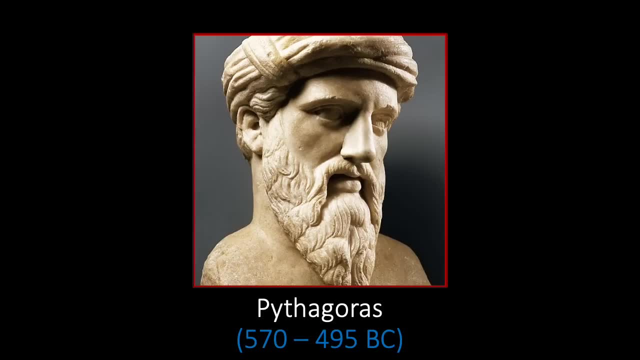 of light came from India and ancient Greece. Many of these theories sought to describe light as a ray, a straight line moving from one point to another. Pythagoras, best known for his theorem of the right-angle triangle, proposed that vision resulted from light rays emerging from a person's 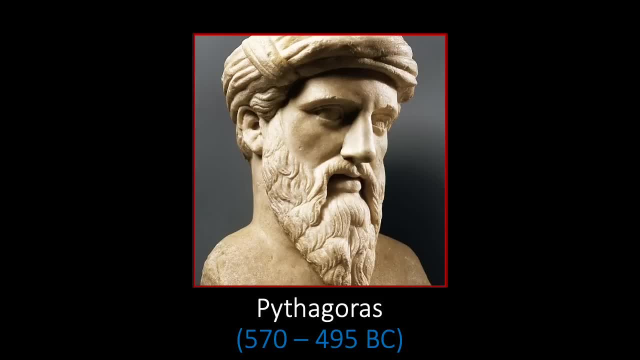 eye and striking an object. Epicurus argued the opposite: Objects produce light rays which then travel to the eye. Other Greek philosophers, most notably Euclid and Ptolemy, used ray diagrams quite successfully to show how light bounces off smooth surfaces. 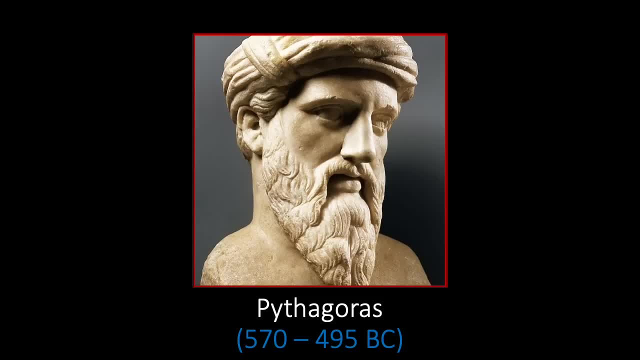 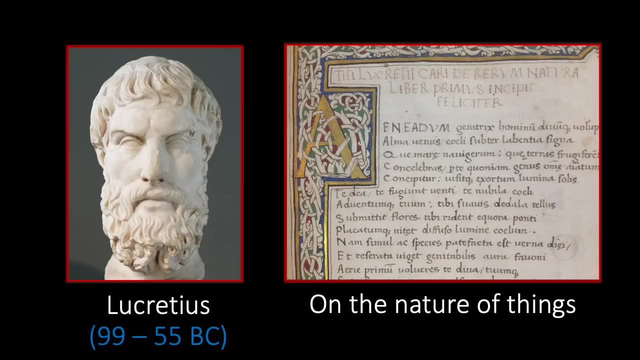 or bends as it passes from one transparent medium to another. Centuries later, Lucretius, who, like Democritus before him, believed that matter consisted of indivisible atoms, thought that light was made of particles travelling in straight lines from the sun. 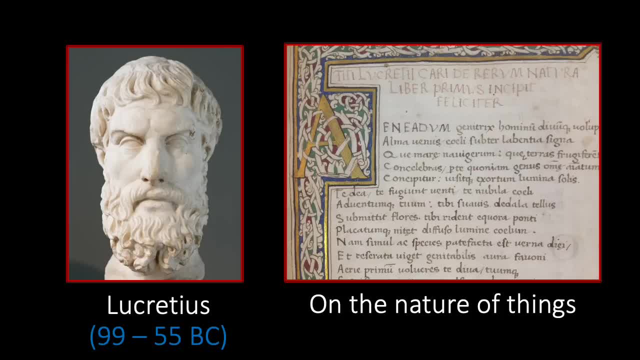 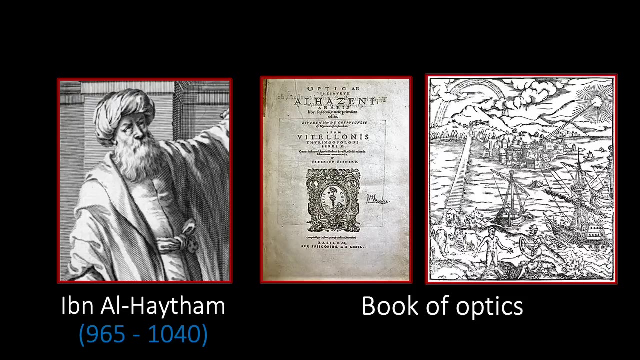 This provided a simple explanation for the formation of shadows. These were just regions in which the light particles couldn't reach, with the sharp edges of the shadows simply representing the boundary between where the particles could and couldn't reach. During the 10th century, the particle theory was developed in Egypt by the famous Middle Eastern. 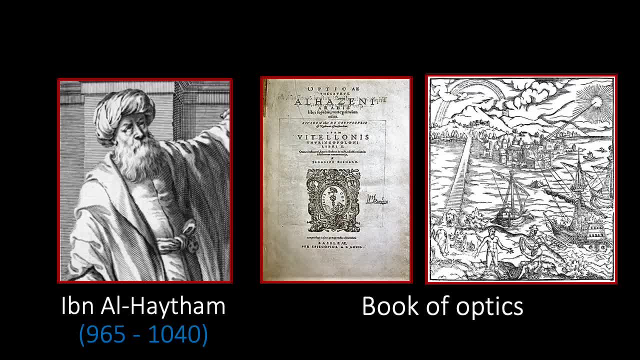 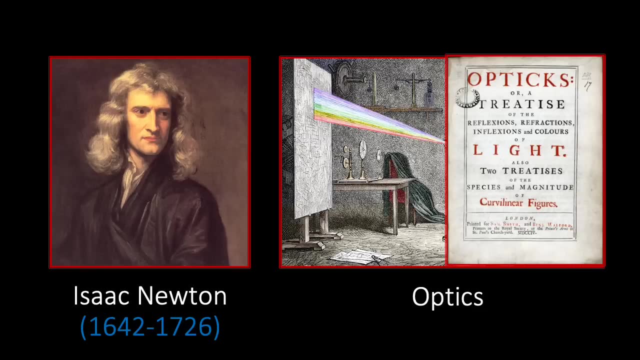 mathematician Ibn al-Haytham, who published a book of optics in 1027, which was the first comprehensive treatment of the properties of light, including the physiological treatment of the eye and the bending and focusing properties of lenses and mirrors. But perhaps the most significant, 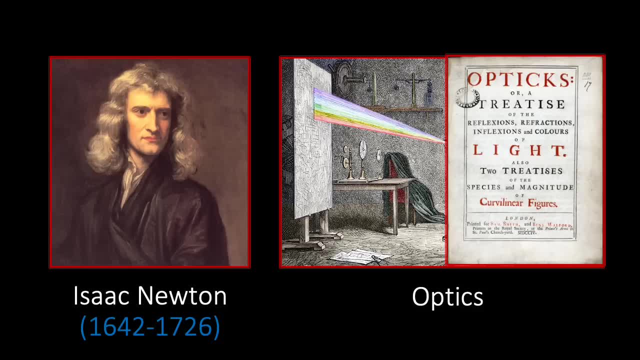 development of the particle theory of light was that of Isaac Newton in the 18th century. Newton showed how reflection, refraction and dispersion could all be explained by the particle theory. According to Newton, light comprised a continuous stream of particles that were given. 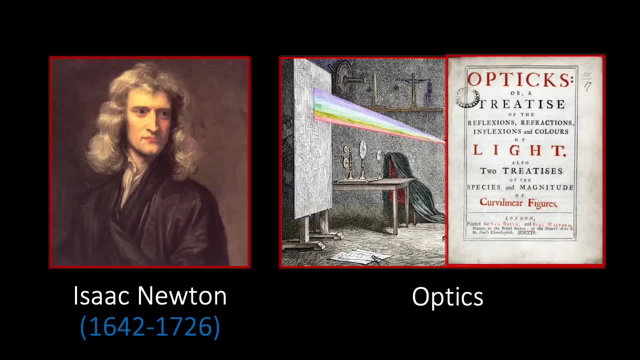 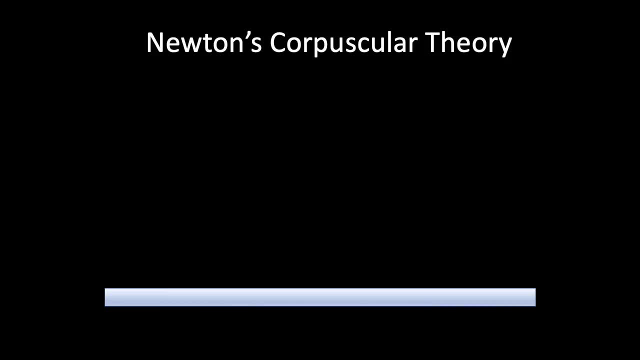 out in all directions by luminous objects. According to Newton, the reflection of light was similar to the reflection of a ball thrown at a hard surface. The ball bounces back at the same angle that it was thrown at. If we considered the initial velocity of the light particle, at some 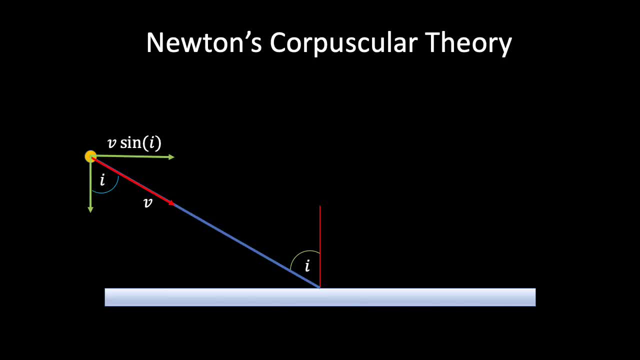 angle i, then we can resolve the velocity into its horizontal and vertical components. As the ball hits the surface, its vertical component of velocity is reversed, but the horizontal component remains unchanged. So we see that v sine i equals v sine r, and therefore sine i equals. 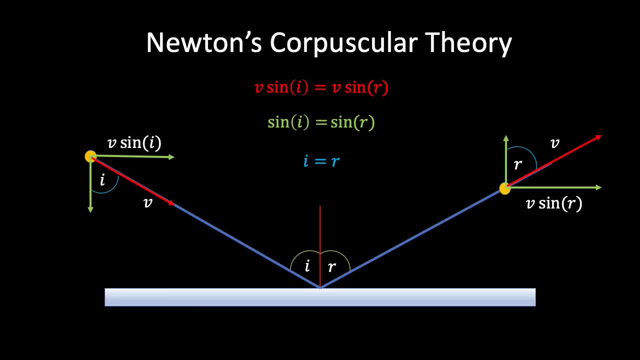 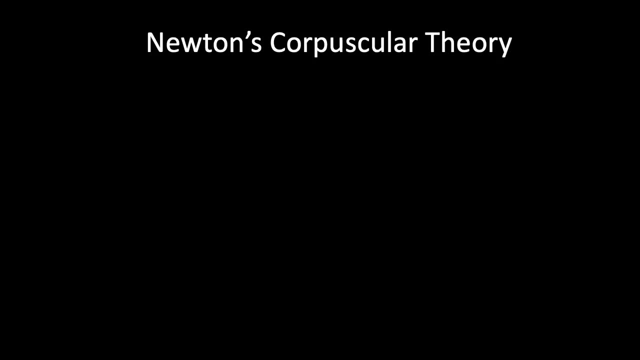 sine r, and so we see that i equals r, The angle of incidence equals the angle of reflection, and the light particle is reflected at the same angle at which it hit the surface, Which we recognise as the famous empirical law of reflection. In order to explain refraction, 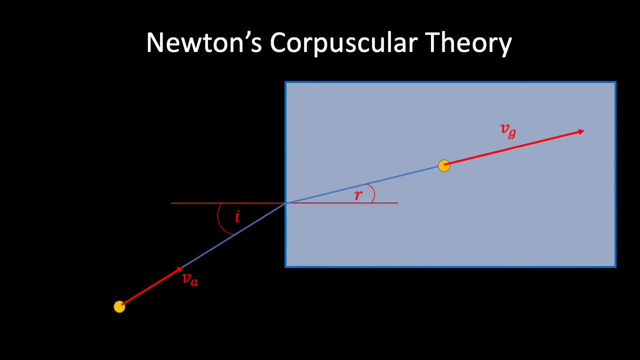 which is the bending of light as it passes from one transparent material into another. Newton assumed that there was a force of attraction between matter and light. According to Newton, when light particles were in the middle of a transparent medium such as air, glass or water, then the forces acting on the particles acted on all sides equally. 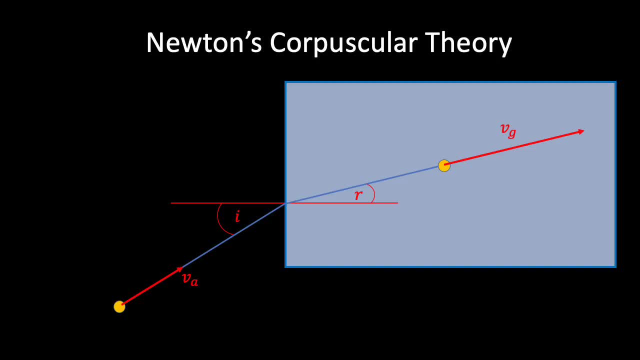 and therefore there was no resultant force. However, if a beam of light is aimed at a glass block, then at the boundary between the air and the glass the forces are unbalanced and there will be a greater force of attraction on the particle towards the glass. This means that the horizontal component of velocity increases. 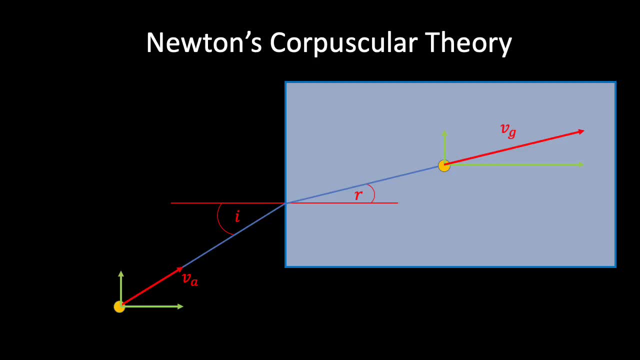 whereas the vertical component remains unchanged. The increase in the horizontal component explains why the light ray changes direction towards the normal on entering the medium. It can also explain the increase in the angle of the light when leaving the medium. However, Newton's particle theory was not without its problems. Firstly, Newton's theory required. 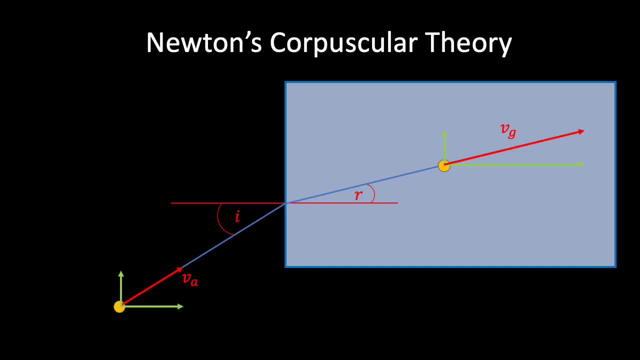 the speed of light to be faster inside a medium than in the air, and this would later be shown to contradict experiment. Secondly, if luminous objects are continuously emitting particles of light, then Newton's theory predicted that the object should be constantly losing mass. And finally, 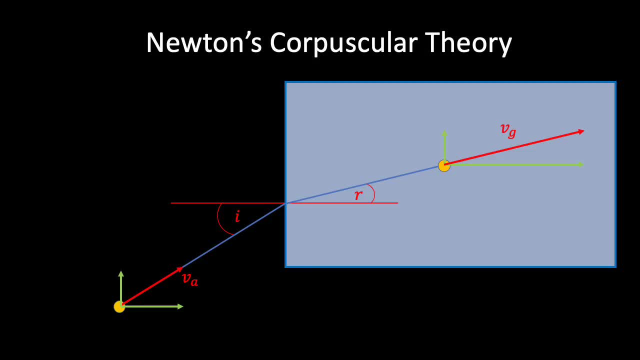 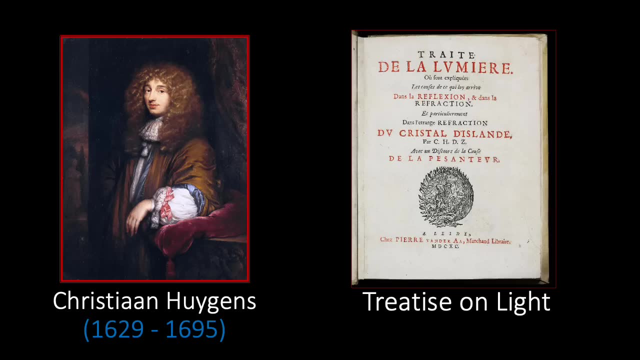 Newton's theory struggled to explain what happens when light passes through a narrow slit and spreads out a phenomenon known as diffraction Around. the same time that Newton was developing his particle theory of light, Christian Huygens, a Dutch astronomer, proposed that light was a 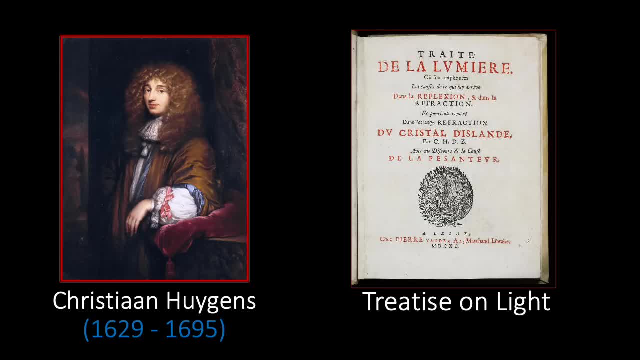 longitudinal wave similar to sound. In much the same way that sound waves require a medium through which to travel, Huygens proposed that longitudinal light waves also require a medium to travel through. Huygens proposed that space was filled with a transparent, massless substance called ether. 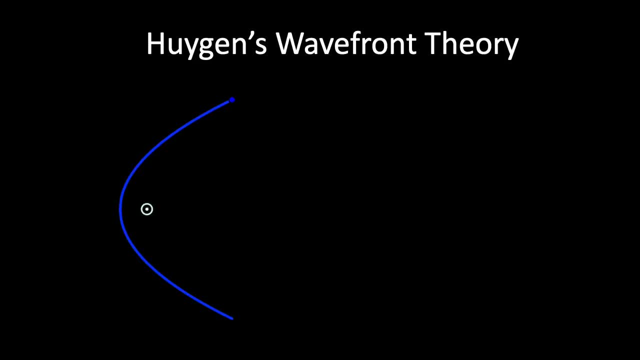 According to Huygens' theory, waves travelled through different materials by the propagation of wavefronts. According to Huygens, each point on the original wavefront acts as a new point source and wavelets spread out from them. These wavelets then combine to form a new wavefront. 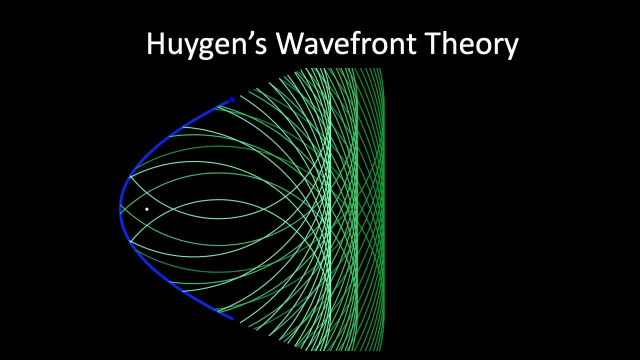 Using the idea of wavefronts, not only was Huygens able to explain the reflection and refraction properties of the new wavefront, but he also was able to explain how the wavefronts and the new wavefronts can form a new wavefront. 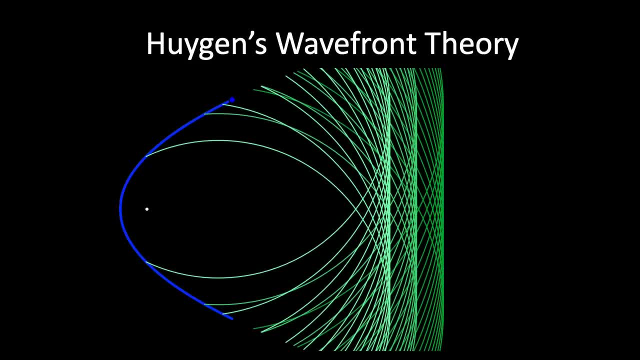 of light. he was also able to explain the diffraction, or spreading out, of light. Despite the success of Huygens' theory, the particle theory of light reigned supreme for over 150 years, largely due to the powerful influence of Newton. After all, Newton's laws. 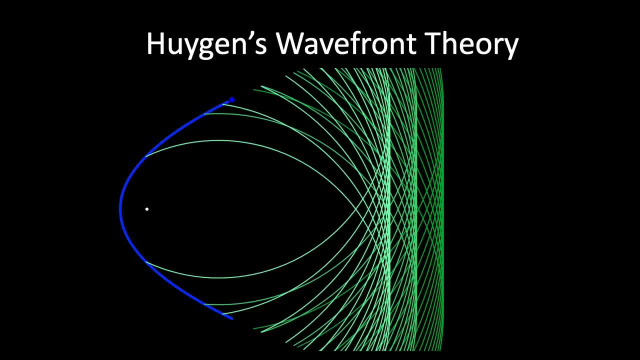 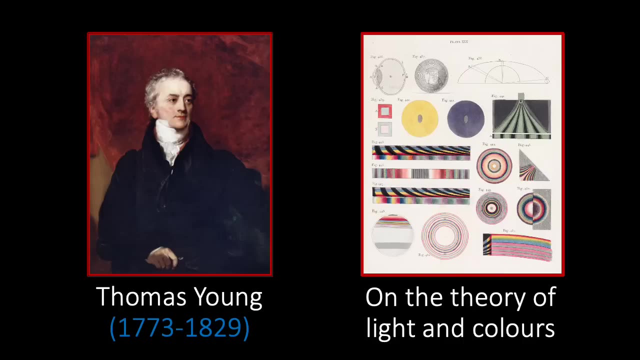 of motion and his theory of gravitation had been so successful at explaining and predicting the future motions of objects that many scientists just assumed that Newton must be correct when it comes to the properties of light. However, when Thomas Young conducted a series of groundbreaking experiments at the beginning of the 19th century, scientists couldn't help but take notice of the 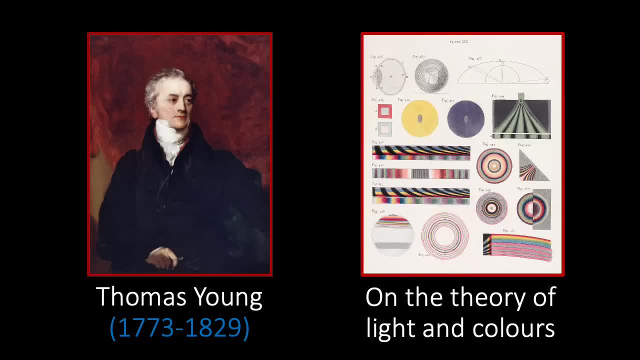 explanatory power of the wave theory of light. In 1801, Young presented a famous paper to the Royal Society entitled On the Theory of Light and Colours, which described the interference properties of light. The first experiment was quite simple and Young wrote: 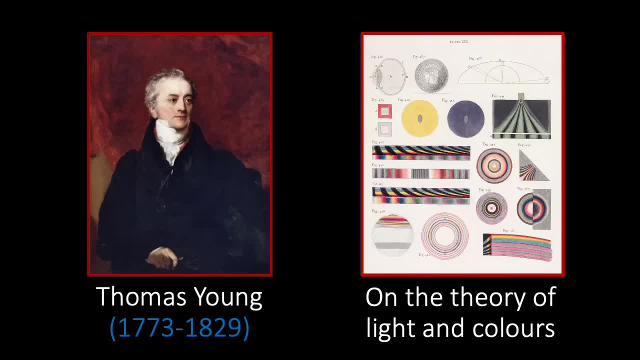 I made a small hole in a window shutter and covered it with a piece of thick paper which I perforated with a fine needle. I brought into the sunbeam a slip of card about one thirtieth of an inch in breadth and observed its shadow. Young described his observations of dark shadows caused by the. 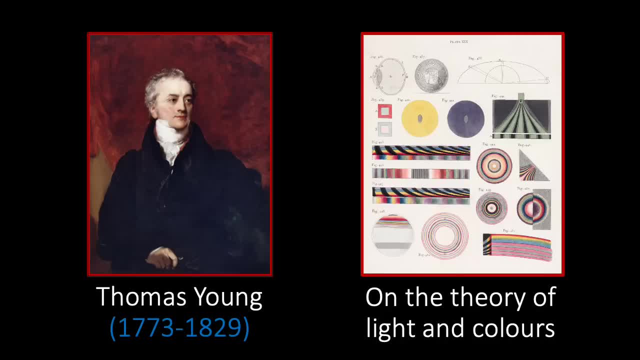 destructive interference of light. by writing. we may infer that a homogenous light at certain equal distances in the direction of its motion is possessed of opposite qualities capable of neutralising or destroying each other, and of course, of course, of the opposite qualities. 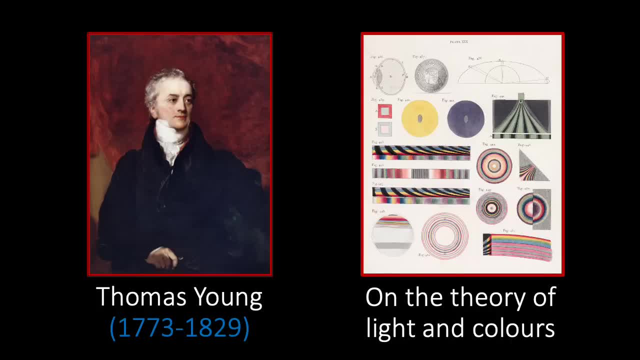 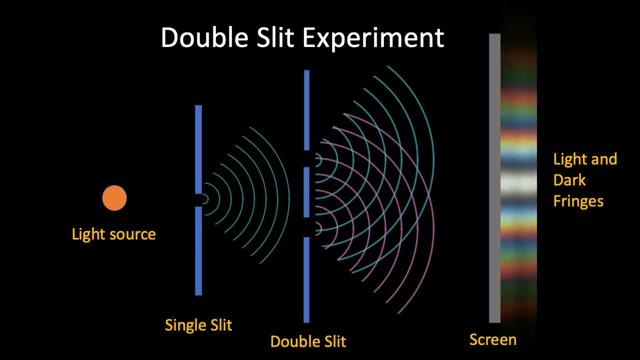 Young was referring to what we now call the principle of superposition, which is a fundamental property of waves. The modern analogue of Young's experiment involves shining a light through a narrow slit so that it spreads out or diffracts. The diffracted light is then used to illuminate. 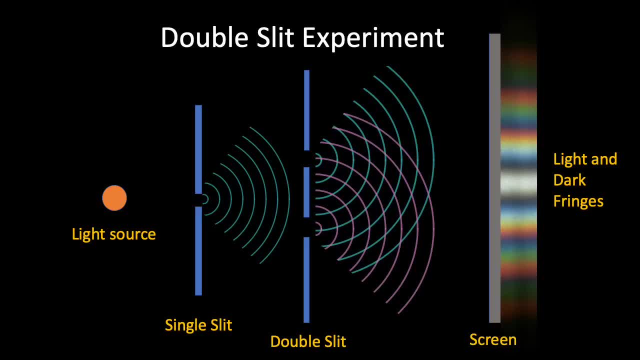 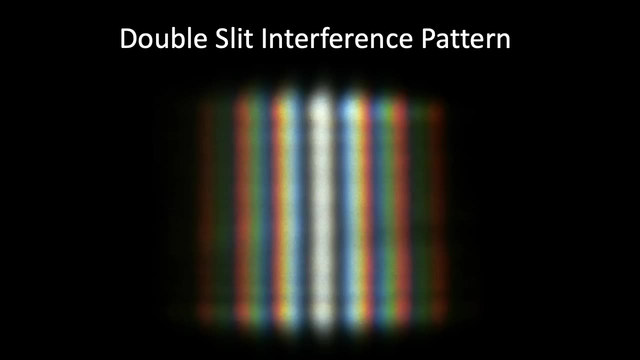 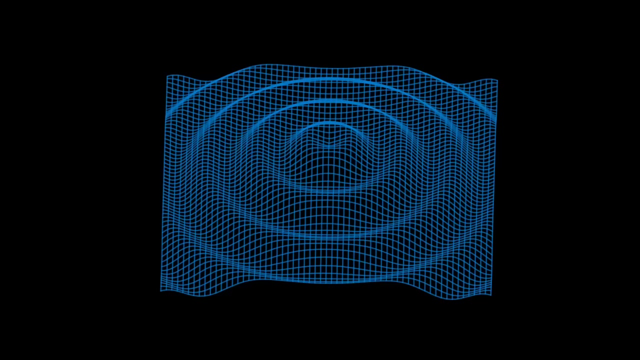 two small parallel slits. Further diffraction at each of these slits causes two sets of overlapping waves which interfere with each other. Young's experiment was called the principle of superposition, which is a fundamental property of waves. Young assumed that light was a wave which propagated through space in much the same way that a water. 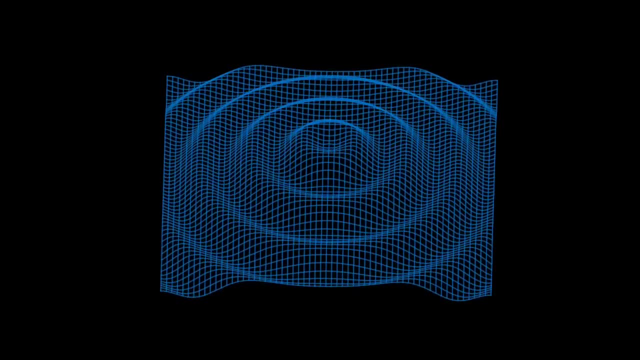 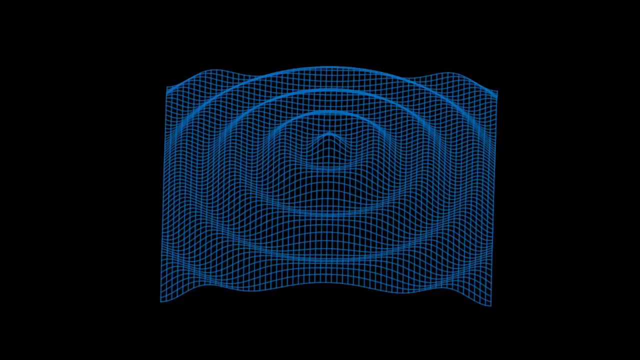 wave moves across the atmosphere. Young assumed that light was a wave which propagated through the surface of water. The distance between adjacent crests is referred to as the wavelength of the wave, and the height of the wave above the equilibrium position is referred to as the 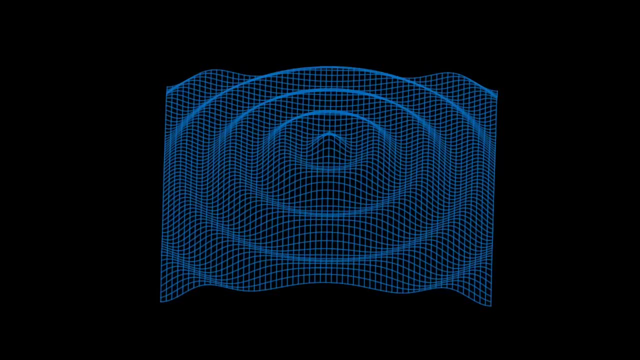 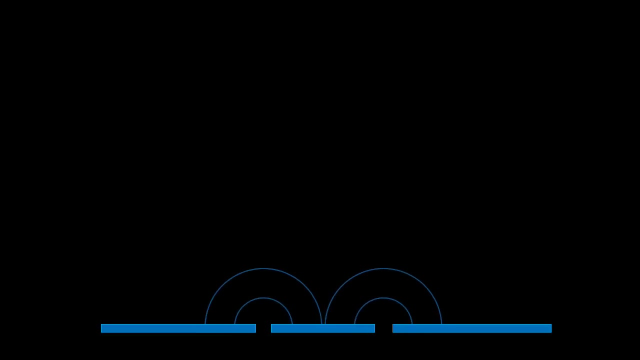 wave amplitude. According to Young, the amplitude of a light wave determines the brightness of the light. The larger the amplitude, the brighter the light. Young was able to use this wave picture to explain the light and dark fringes When the light falls upon the two narrow slits. 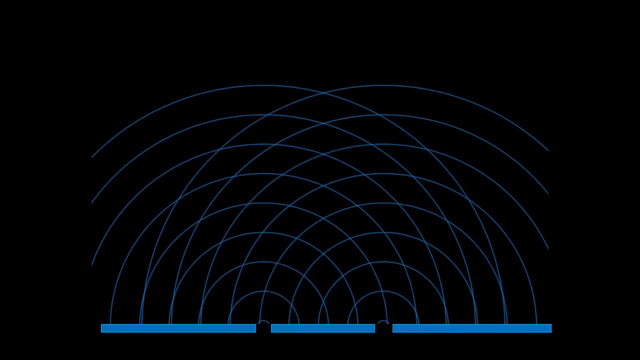 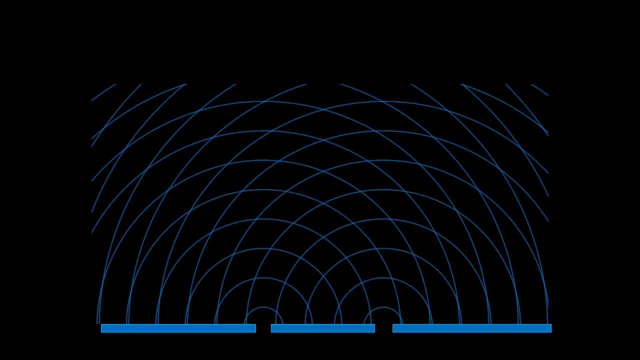 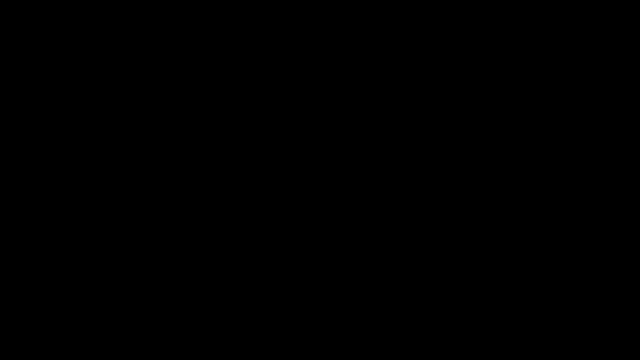 it diffracts at each slit and spreads out. The two sets of diffracting waves overlap one another in space. If two waves meet at a point in space, then the net displacement of these two waves will be equal to the sum of the individual displacements at that point. In other words, if a peak of a wave 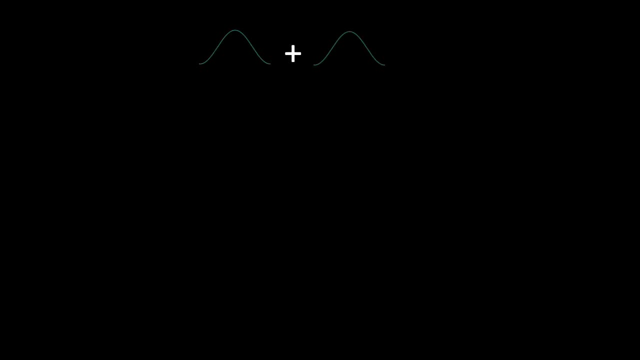 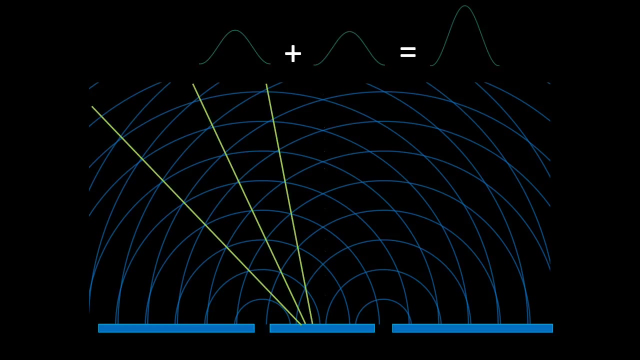 from the first slit encounters a peak of a wave from the second slit, then these two waves will add together, reinforcing one another, to produce a large amplitude peak corresponding to the amplitude of the first slit. We see from the diagram that this will occur along each of the following lines: 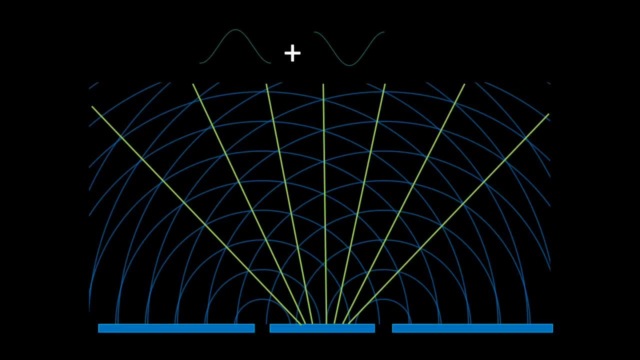 If, on the other hand, a peak encounters a trough, then these two waves could cancel, resulting in a net displacement of zero, which would correspond to no light or a dark fringe, as Young had observed. We see from the diagram that dark cancellation of the two sets of waves. 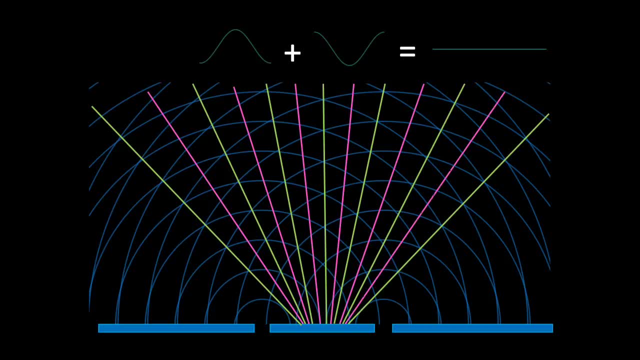 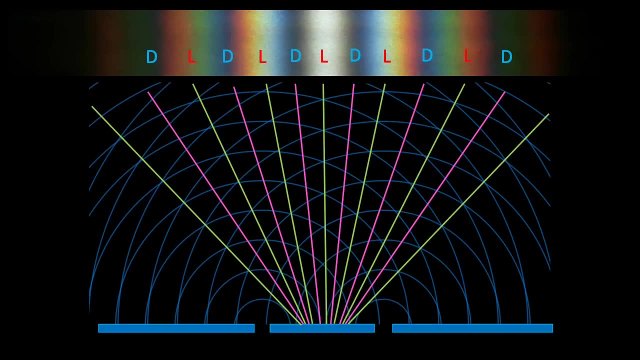 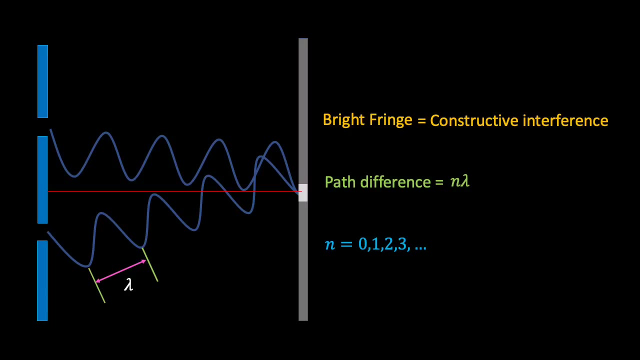 will occur along the following lines. So we see that the pattern of light and dark fringes can be explained using the wave theory of light and the principle of superposition. To understand the double slit interference pattern a bit more quantitatively, we need to consider the paths of the two sets of waves travelling. 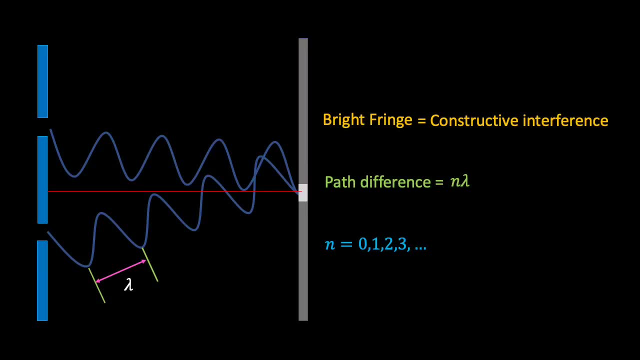 from the slits to the screen. Each slit is a different distance from a given point on the screen. Thus different numbers of wavelengths fit into the different slits. So we can see that the difference in length between the two paths to a point on the screen is equal to a whole number of. 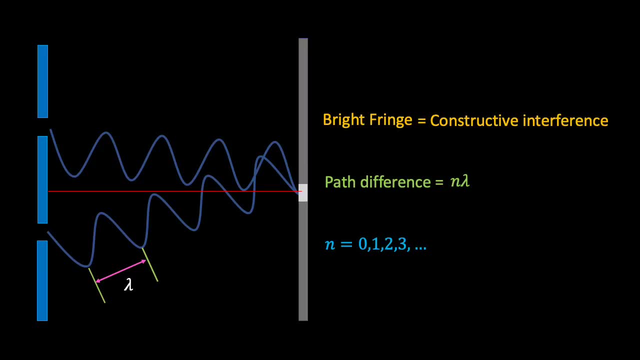 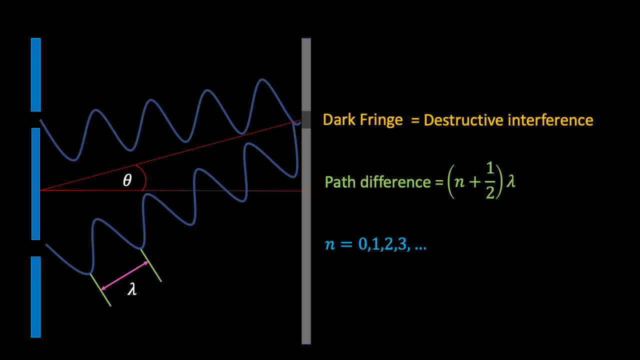 wavelengths, then the waves will arrive at the screen in phase or crest to crest, producing a bright fringe. If, however, the paths differ in length by half a wavelength, then the waves will arrive at the screen out of phase or peak to trough, causing destructive interference which will result. 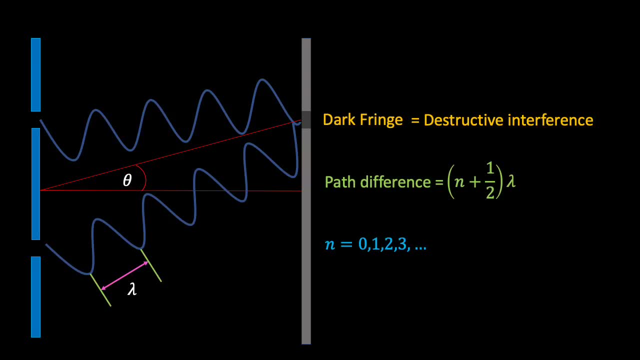 in a dark fringe. These observations of superposition and wave interference supported the earlier work of Huygens and could not be explained by Newton's particle theory of light, signalling a major blow to the particle picture of light and a major success for the wave theory. But 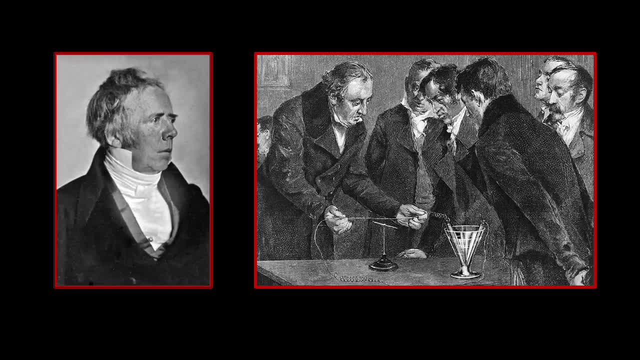 the story didn't end here. Towards the end of the 18th century, physicists had begun to realise that there was a deep connection between electrical and magnetic phenomena. The first documented account of this link occurred in 1820, during a lecture by the physicist Hans 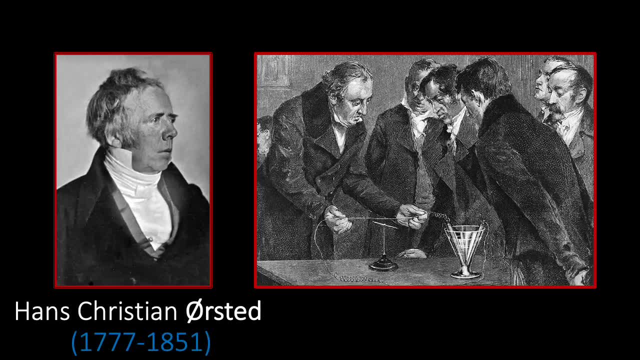 Ørsted For one of the demonstrations in the lecture. Ørsted had a wire connected to a battery. During the lecture he noticed that a compass needle near the wire spontaneously moved away from magnetic north when the battery was connected or disconnected from the wire, Although Ørsted did. 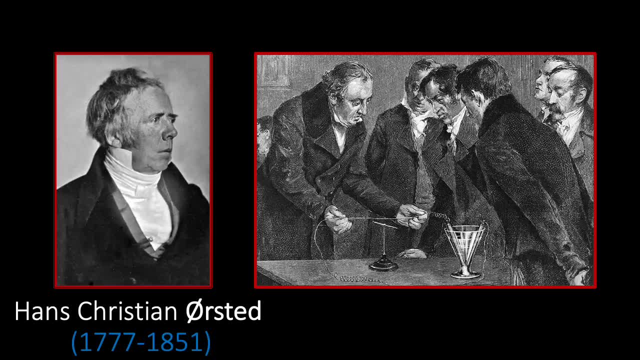 not realise it at the time. this demonstration showed that there was a deep connection between the changing electric current caused by the connection and disconnection of the circuit and the creation of a magnetic field surrounding the wire. However, the nature of the relationship between the two was not clear. 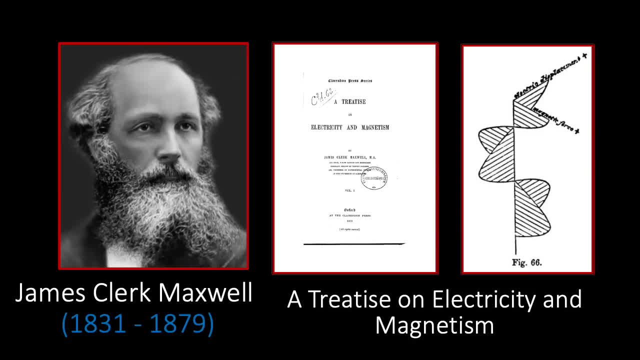 In 1864, James Clerk Maxwell published a paper in which he gave a mathematical description of the relationship between electric and magnetic fields. Not only did his equations account for all observed electric and magnetic phenomena, his equations also predicted that waves of oscillating electric and magnetic fields should exist with a speed that could be calculated. 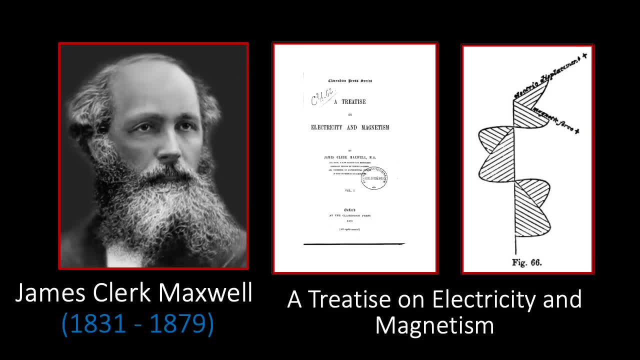 using the measured constants of the theory. Using the measured values of these constants from experiments, Maxwell obtained a value of 300 million metres per second. Comparing this value with the recently measured values for the speed of light, Maxwell wrote: The agreement of the results seems to show that light and magnetism are affections of the same. 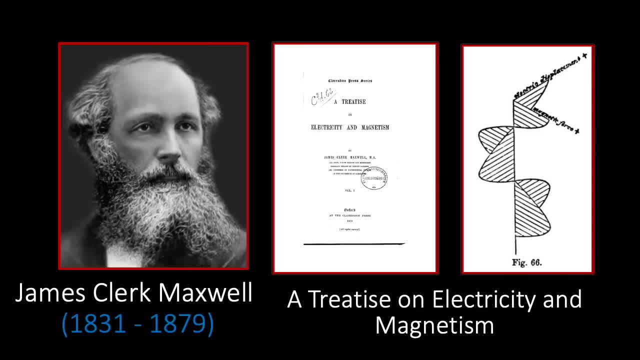 substance and that light is an electromagnetic disturbance propagated through the field according to electromagnetic laws. Maxwell quickly realised that if the speed of light was constant, then there must exist a whole spectrum of wavelengths and frequencies of these newly discovered electromagnetic waves, And by the end of the 19th century both radio waves and x-rays had been discovered. 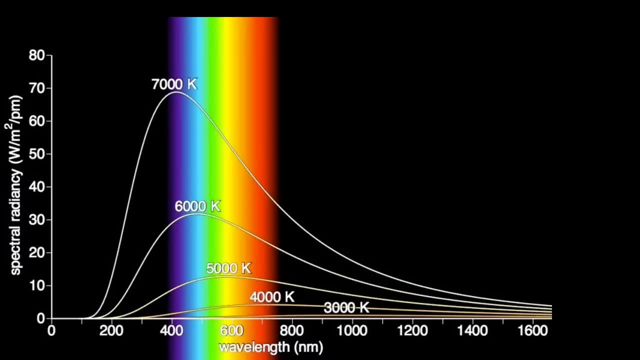 At the turn of the 20th century, it appeared that physics was divided in two. Firstly, you had the physics of matter, based on the concept of atoms, which was supposed to obey Newton's classical laws of mechanics, And secondly, you had light and radiation more. 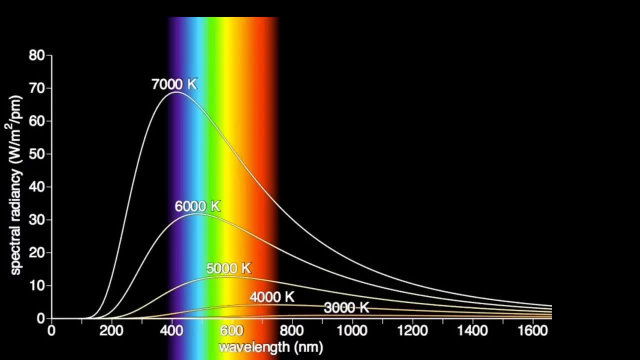 generally, which, in large part due to the work of Young and Maxwell, was based on the concept of wave propagation in a hypothetical medium known as the aether. However, these two realms of physics could not remain alien to each other forever If physicists wished to understand the 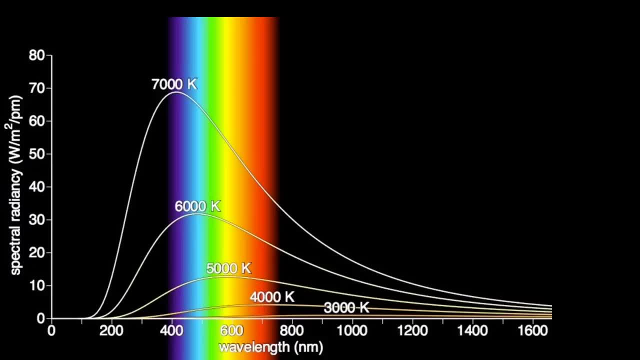 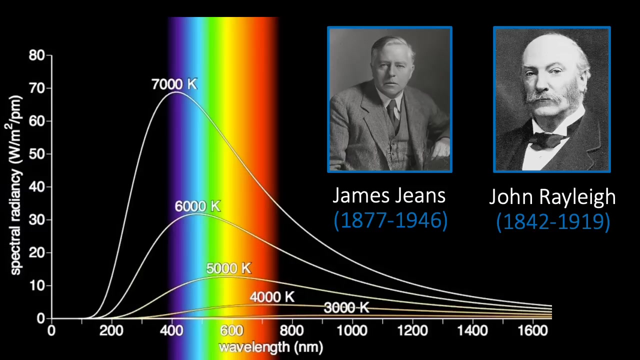 radiation properties of luminous material objects comprised of atoms, they would have to explain the energy exchanges between matter and radiation, And that is where the next set of difficulties arose. In attempting to explain the radiation properties of hot objects, John Rayleigh and James Jeans had combined the newly discovered electromagnetic theory with the well-established 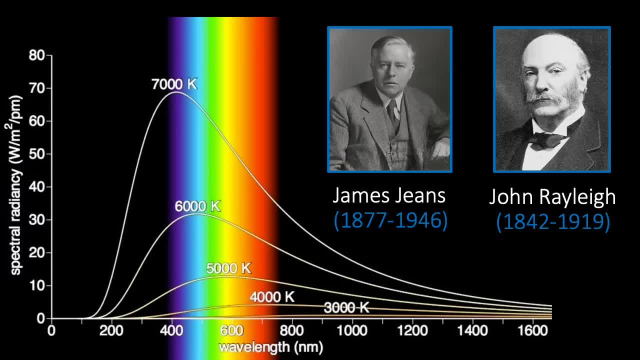 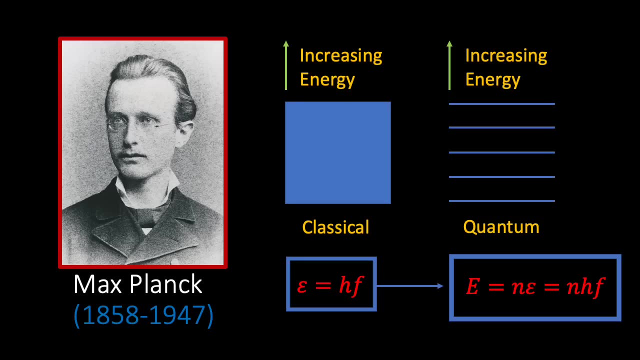 statistical laws of thermodynamics. However, to their alarm, they found that their theory predicted that hot objects should be emitting an infinite amount of radiation At high frequency. So serious was the problem that it was dubbed the ultraviolet catastrophe. The solution to the problem was provided by Max Planck who, in an act of desperation, 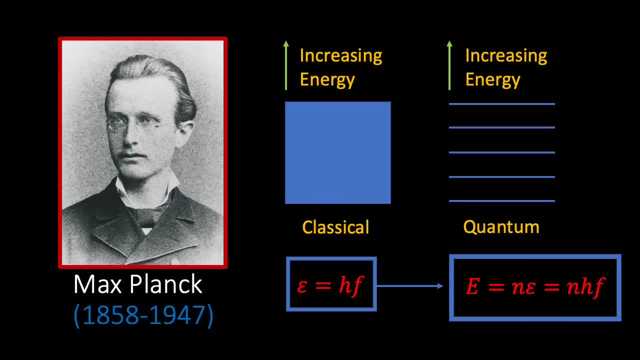 realised that, instead of assuming, in common with the classical wave theory, that energy is transferred continuously, he assumed that it was transferred discreetly in chunks or quanta, with the energy of each quantum being proportional to the frequency f of radiation. In this way, Planck was able to tame the infinities of the ultraviolet catastrophe. 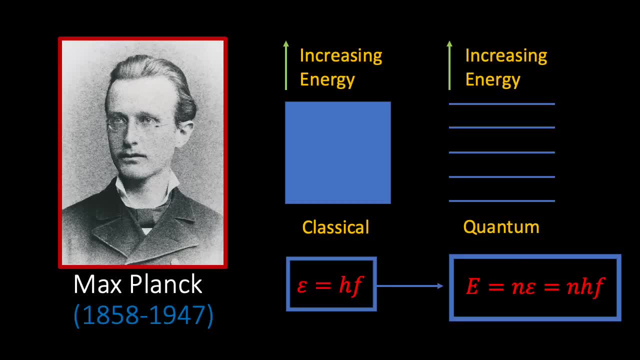 and account for the radiation properties of hot objects. However, the success of Planck's ideas entailed serious consequences. If energy is quantised, then surely light, which carries energy, should be quantised too. Perhaps Newton was right all along, and light is comprised of particles. 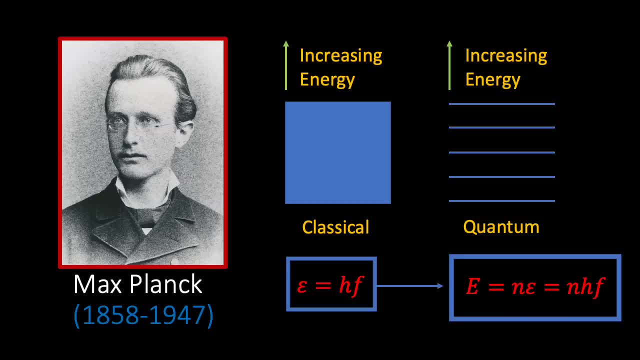 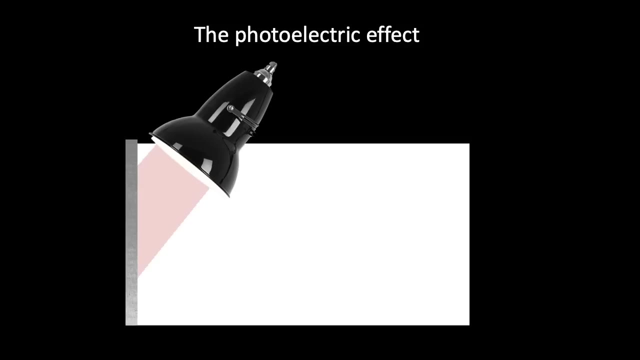 after all, In 1905, the existence of a granular structure of light and of other radiations was confirmed by Einstein's explanation of the photoelectric effect. So what is the photoelectric effect If a beam of light above a certain threshold frequency? 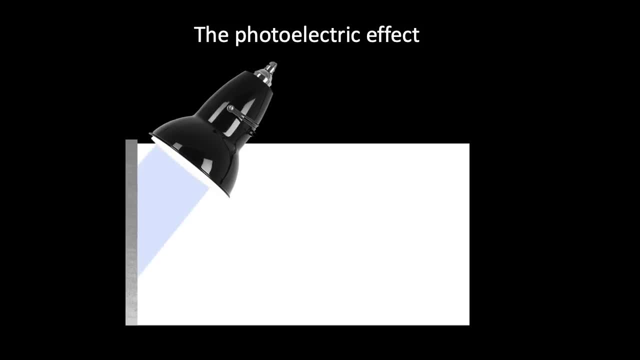 falls onto a metallic surface. electrons are emitted from the surface of the metal with the kinetic energy that increases as the frequency of the light is increased. If, however, the frequency of the light incident upon the metal surface has a frequency less than the threshold frequency, then no electrons will be emitted, no matter how bright or intense the 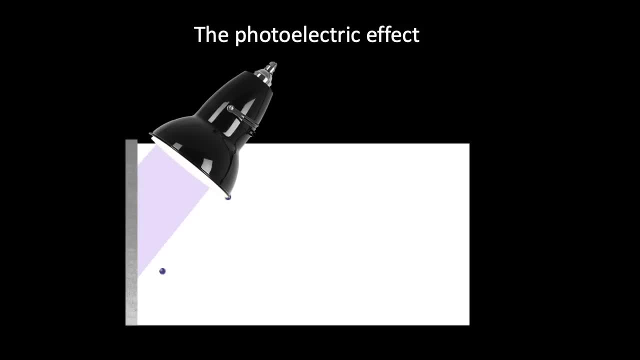 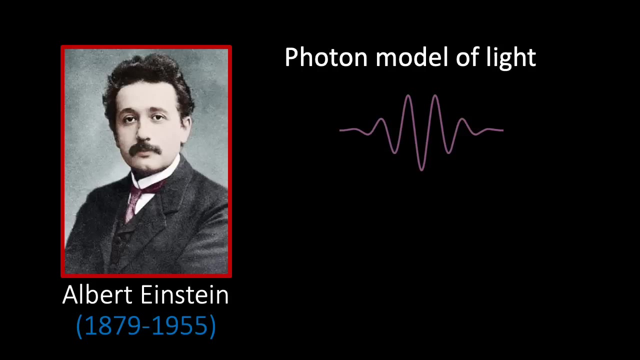 light. This observation could not be explained by the wave theory, which predicted that at low frequencies electrons should still be emitted. The photoelectric effect was explained by Einstein in 1905 by simply assuming that light is composed of tiny particles called photons, each with energy. 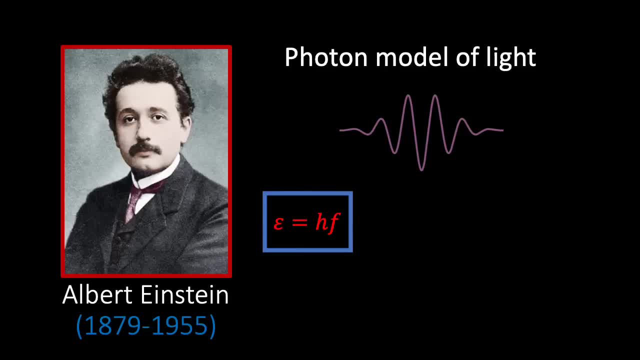 Hf, where f is the frequency of the light and f is the frequency of the light. H is Planck's constant. As the frequency of the light source increases, so too does the energy of each individual photon. When a photon encounters an electron in the metal, the electron absorbs. 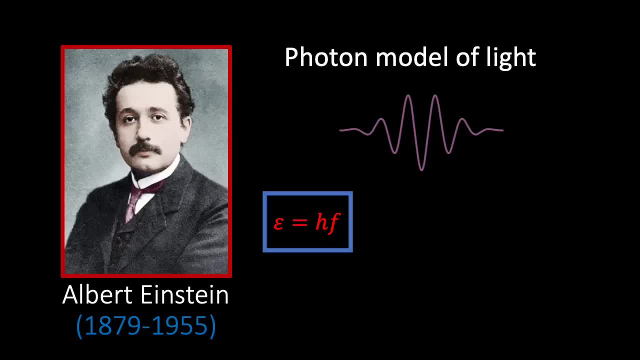 the energy of the photon, and if this energy is greater than the binding energy holding the electron to the surface, phi, the electron is liberated and leaves the surface with any excess energy, providing the kinetic energy of the electron. This simple yet powerful explanation. 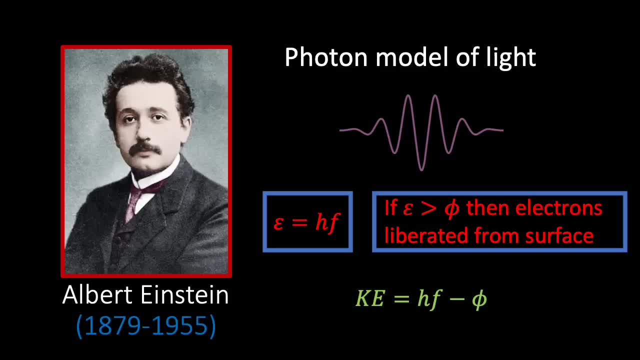 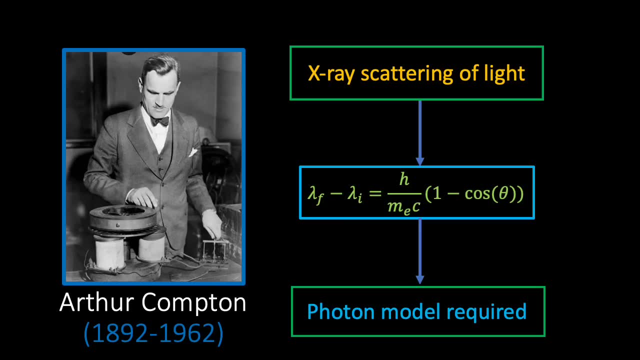 of Einstein's would not only win him the Nobel Prize but provide the most compelling evidence yet for the particle nature of light. However, it would still take a further 17 years until Arthur Compton's explanation of x-ray scattering using the photon model of light finally convinced the 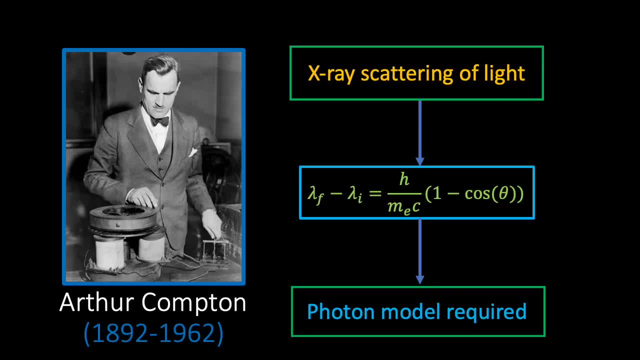 physics community that the particle model needed to be taken very seriously. Yet despite the success of the photon model, it was still necessary to explain the particle nature of light. The photon model of light was not necessarily necessary to adopt the wave theory to account for the 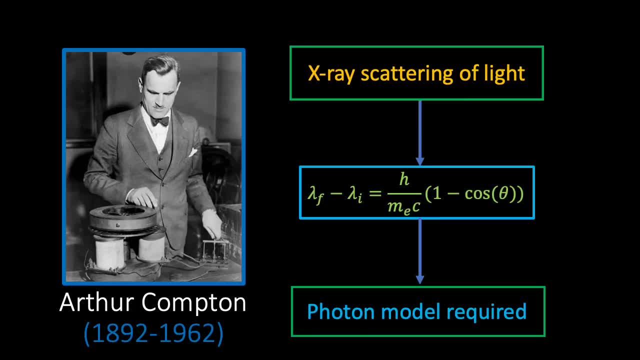 interference and diffraction phenomena of light, and no way whatsoever of reconciling the wave theory with the existence of light particles could be visualised. Physicists at the time were only half-joking when they complained about having to teach wave theory of light on Mondays, Wednesdays. 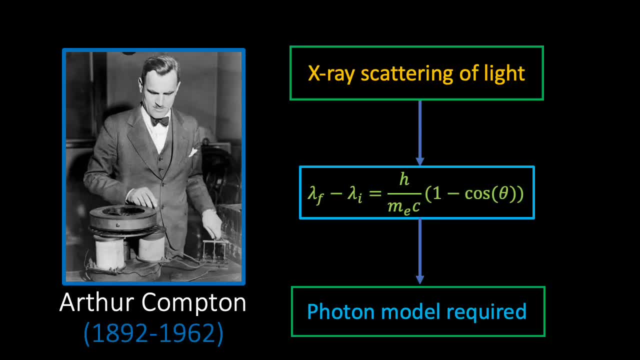 and Fridays, and the particle theory on Tuesdays, Thursdays and Saturdays. What was needed was a new unified vision of atomic physics, one capable of detecting the particle and wave pictures. This new vision would be provided by Prince Louis-Victor. 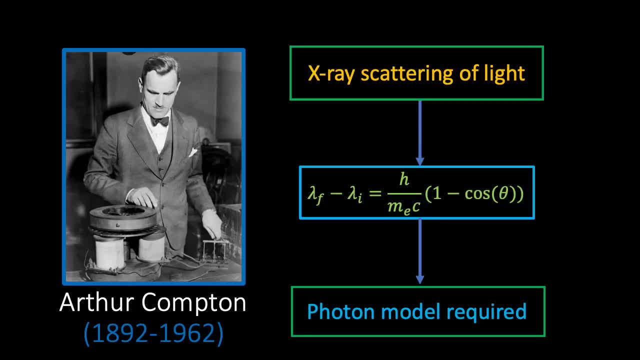 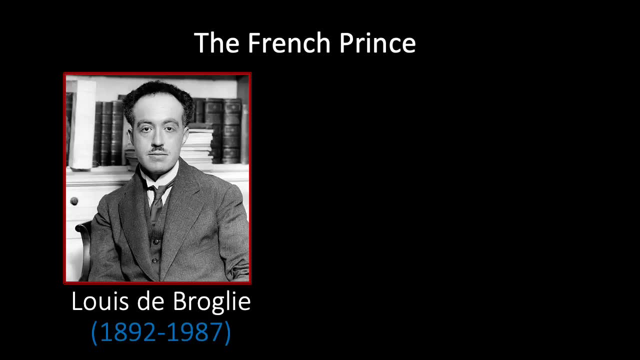 Pierre-Raymond de Broglie, a member of one of France's leading aristocratic families. The youngest of four, Louis, was born in Dieppe on the 15th of August 1892.. In 1913, after abandoning his study of history in favour of physics, in large part due to his 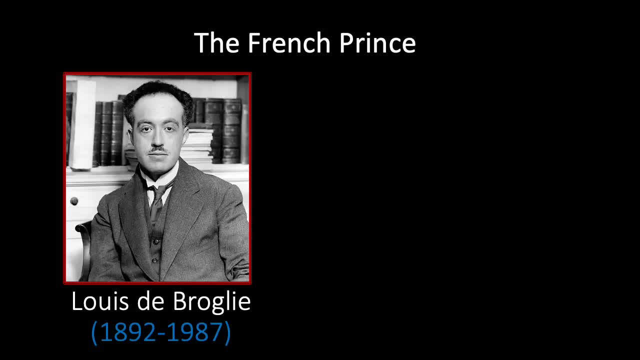 older brother's enthusiasm about his own research into x-ray phenomena, he was awarded his degree, One year of military service beckoned. however, the outbreak of the First World War meant that he was only discharged from service in 1919, having spent the majority of his time working in the field of. 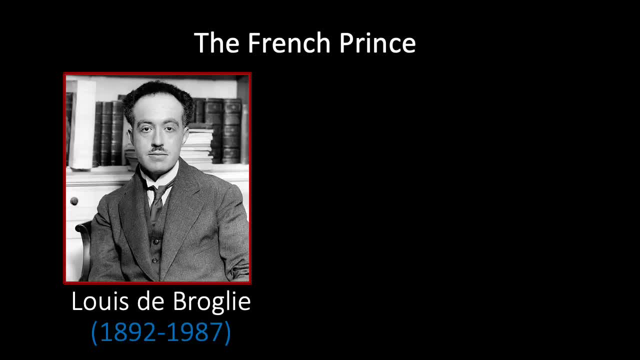 wireless communications as a radio engineer underneath the Eiffel Tower. Now aged 27,, de Broglie was more determined than ever to continue his study of physics, Initially working in his brother's laboratory, he published a few papers on the absorption of x-rays whilst thinking. 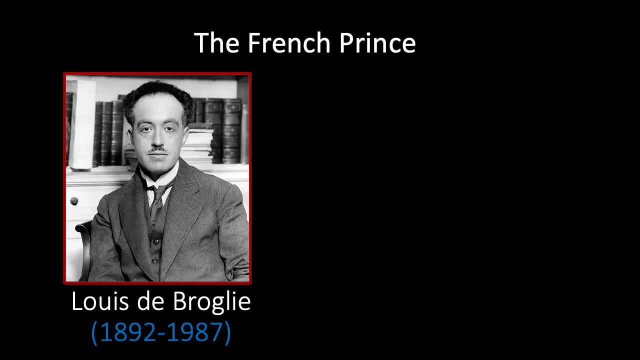 about the nature of electrical energy. He was also a professor at the University of Paris- an electromagnetic radiation. Both he and his brother accepted that both the wave and particle theories of light were in some sense correct, since neither on its own could explain both diffraction and 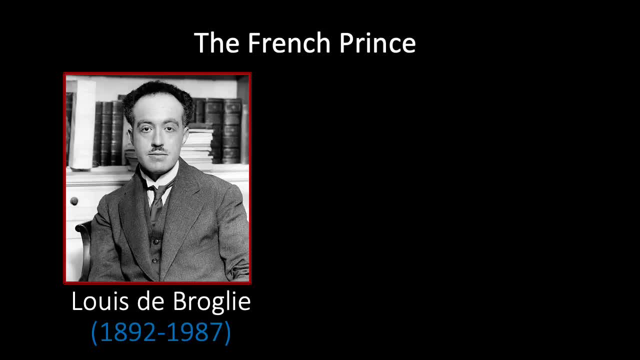 interference and also the photoelectric effect. When de Broglie started to seriously ponder the dual properties of light, two things struck him. Firstly, the light quantum theory cannot be regarded as satisfactory, since it defines the energy of a light particle by the relationship. 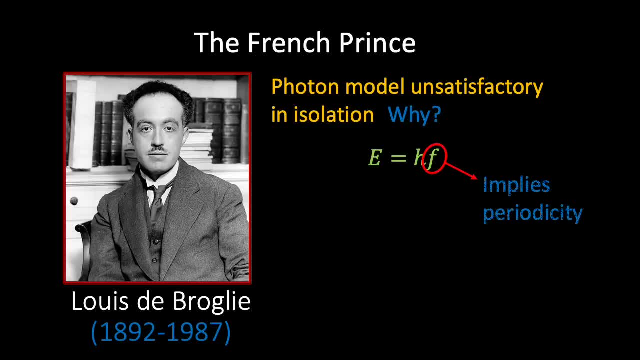 E equals hf, which contains a frequency. f Now, a purely copuscular theory, does not contain any element permitting for the definition of a frequency. This reason alone renders it necessary, in the case of light, to introduce simultaneously the particle concept and the concept of periodicity. 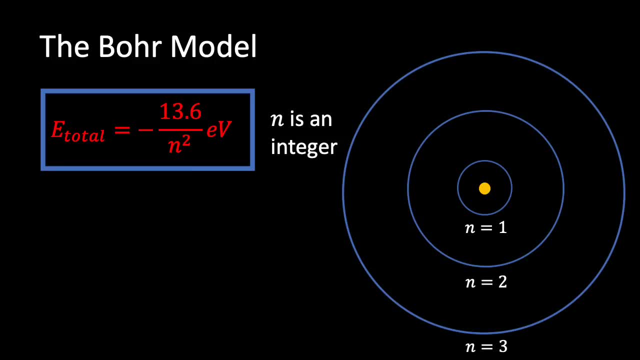 Secondly, Niels Bohr had shown that the determination of the energy levels of electrons inside the hydrogen atom involves whole numbers, with the energy levels being determined by the principal quantum number, N, with N being an integer. According to Bohr's model, only certain discrete energy 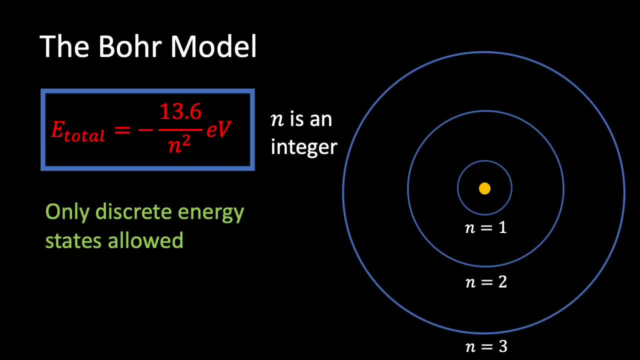 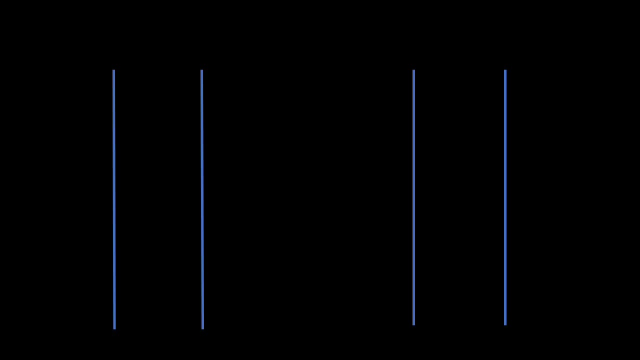 levels are permitted inside the atom. As far as de Broglie could tell, the only other phenomena in which whole numbers played such a central role were those of wave interference in stationary wave patterns. If a string which is fixed at both ends is plucked, then only certain discrete 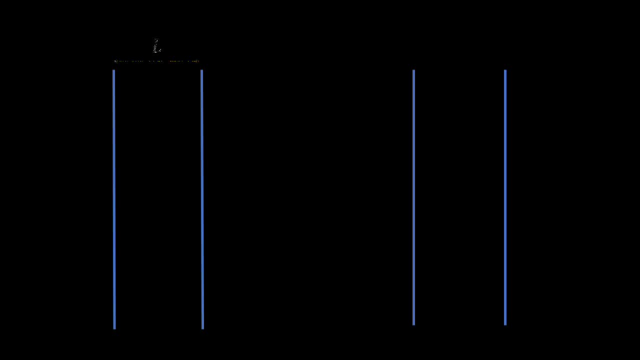 wavelengths are permitted. If the length of the string is L, then we see that the first mode of vibration is the length of the string. If the length of the string is L, then we see that the length of the string is L. If the length of the string is a wavelength equal to 2L, the second mode has wavelength L, the third mode has wavelength 2L over 3, and. 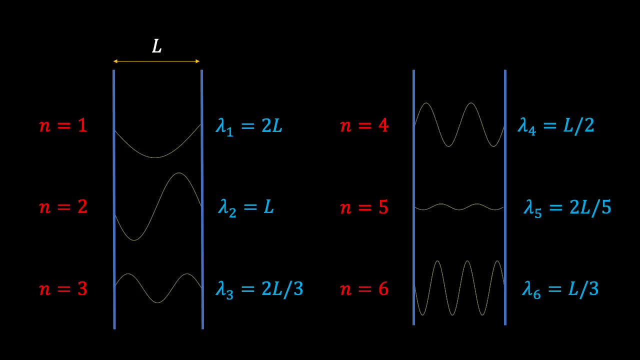 so on. In general, only an integer number of half-wavelengths are able to fit between the two fixed ends, and the wavelength of the nth mode of vibration is given by 2L over N, where N is an integer. It was the discrete nature of the possible vibrational modes that reminded de Broglie of the energy. 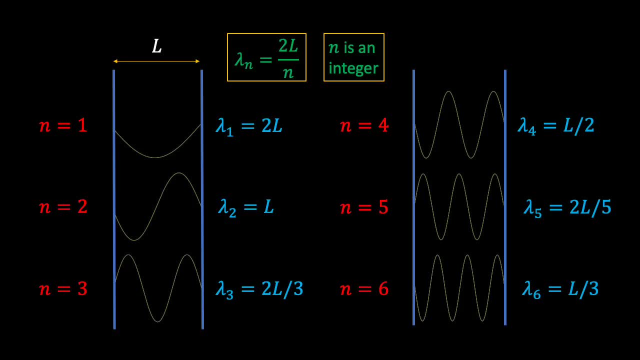 levels inside Bohr's atom. This led de Broglie to the idea that electrons themselves could not be represented as simple particles either, but that a periodicity had also to be assigned to them, just like with the photons of light. Thus de Broglie arrived at the following overall concept: 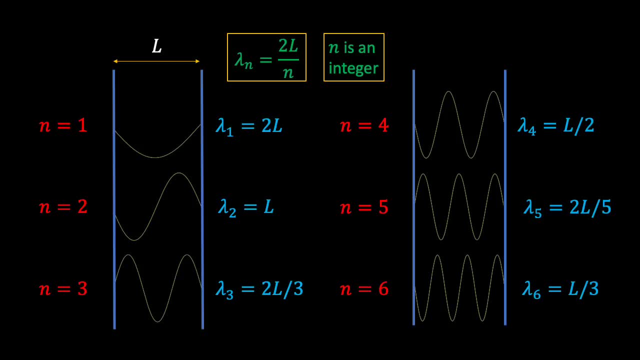 which guided his studies. For both matter, and radiation light in particular, it is necessary to introduce the particle concept and the wave concept at the same time. In other words, the existence of particles accompanied by waves has to be assumed in all cases. De Broglie had dared to. 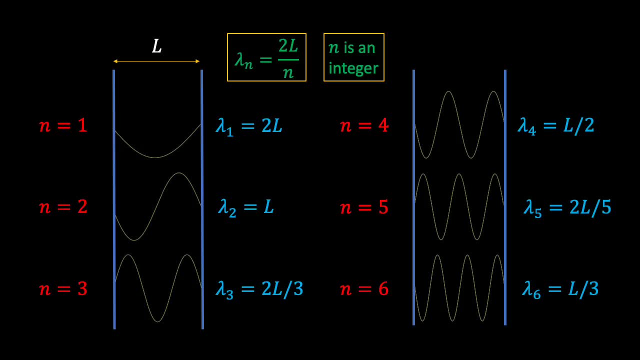 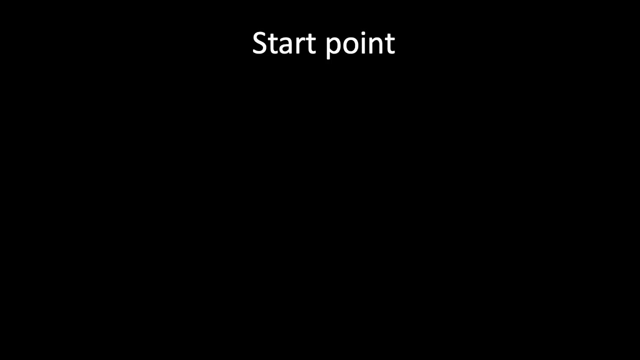 ask the question if light waves can behave like particles, can particles such as electrons behave like waves? De Broglie's answer to his own question was an unequivocal yes. De Broglie's start point was Einstein's 1905 paper on the photoelectric effect. According to Einstein, the energy of a photon, which is one of 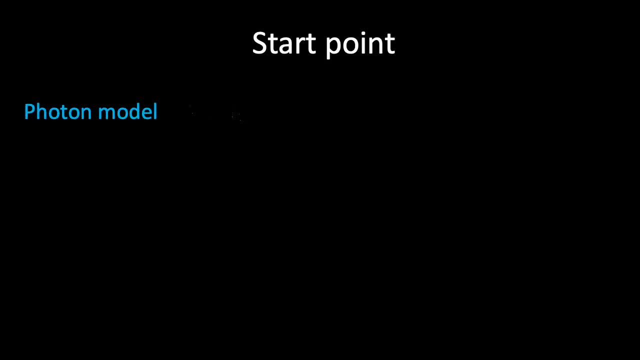 the defining properties of a particle is given by the equation E equals hf, And if we combine this with the relationship linking the speed of light with the wavelength and frequency of light, then we can write E equals hc over lambda. But Einstein also proposed that these little particles of light 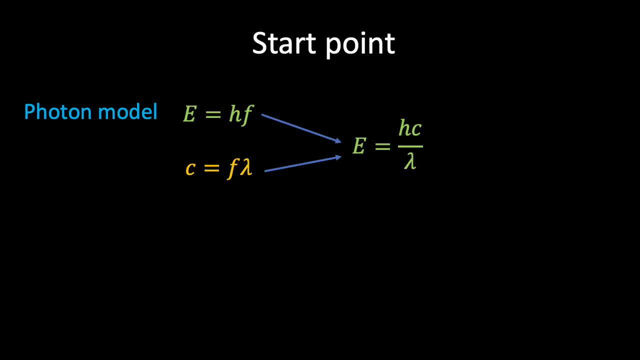 carry momentum as particles should. Now it might seem counterintuitive to assign momentum to a massless particle of light, since according to classical physics, we define the momentum of a particle as p equals mv, so we should expect a massless particle to have zero momentum. However, according to Einstein's special theory of, 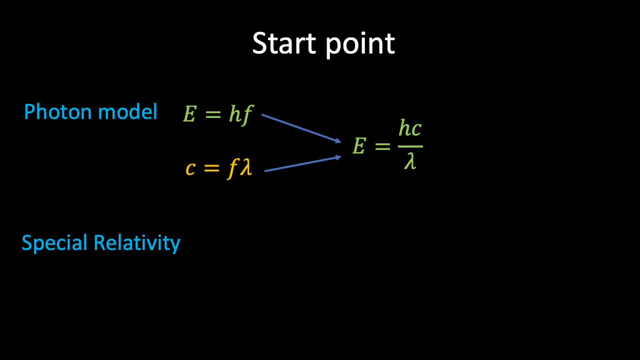 relativity, the total energy of a particle is given by the expression: E squared equals p squared c squared plus m, naught, c squared. So the total energy of a particle is given by the expression: E squared equals p squared, c squared, plus m, naught, c squared. 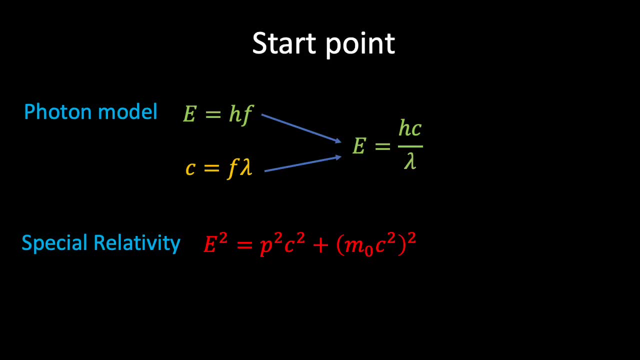 squared, all squared. where m naught is the rest mass or the mass of the particle. and we see from this relativistic expression that if m is equal to zero, we find that p equals e over c and therefore, if we combine this with the equation e equals hc over lambda, we finally arrive at the expression. 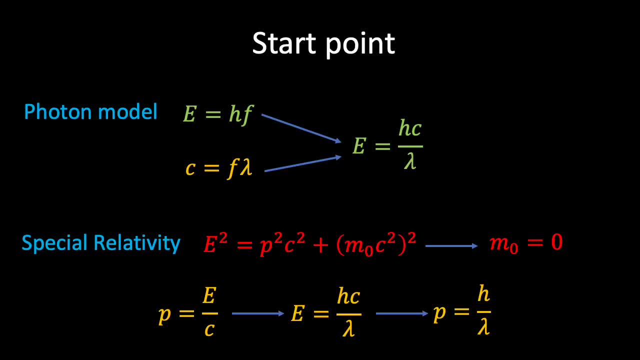 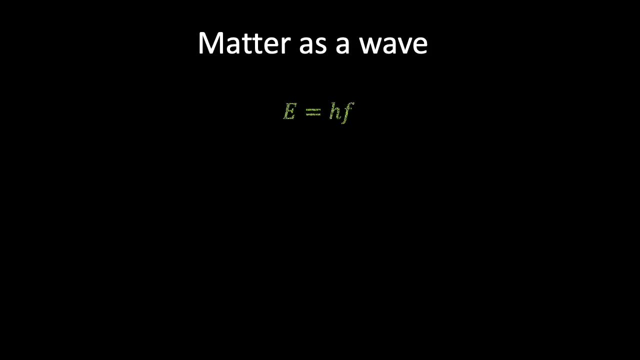 p equals h over lambda, And so we see that Einstein's photon model links particle and wave properties via two equations: e equals hf and p equals h over lambda. Here the particle concepts- energy and momentum- are connected via Planck's constant to the wave concepts frequency and. 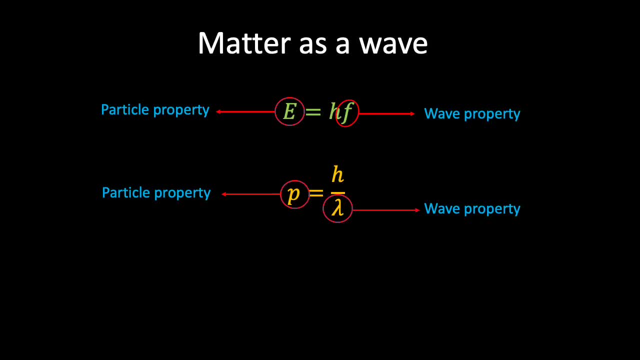 wavelength. Now what de Broglie did was simply assume that these two relationships hold for all momentum. De Broglie proposed that for a matter particle with momentum p, you can associate a plane wave of wavelength lambda equals h over p. This equation predicts the de Broglie wavelength. 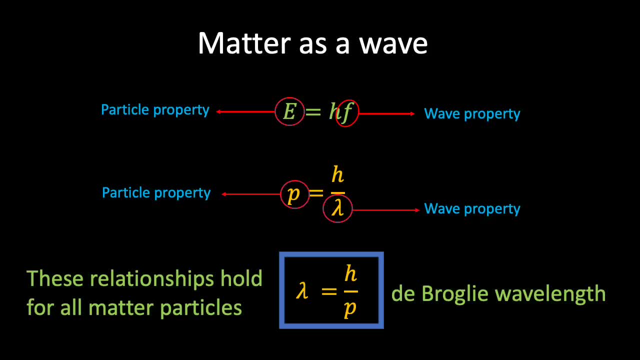 of a matter wave associated with the motion of a material particle with momentum p, Although there was no experimental evidence at the time to support de Broglie's hypothesis, he was encouraged by the fact that he was able to provide an experimental evidence to support de Broglie's hypothesis. 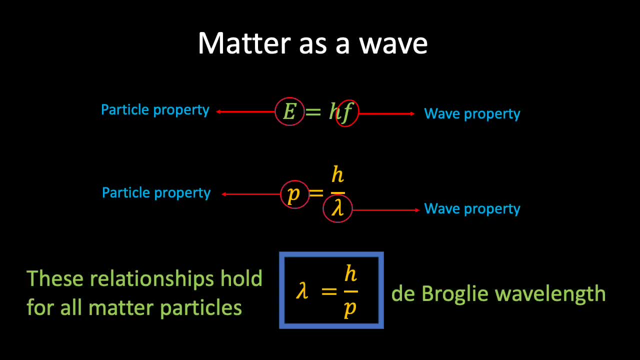 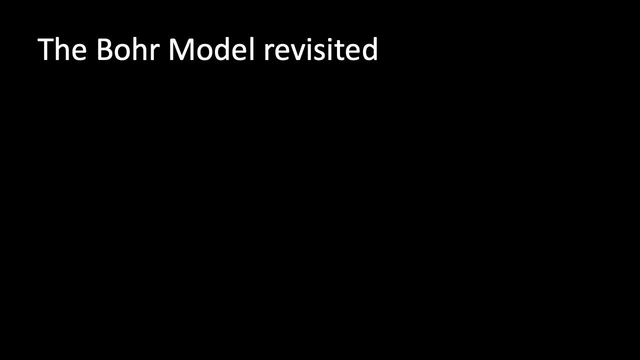 This is an explanation for Bohr's model of the atom. using the matter wave hypothesis. Recall that in 1913, in order to stabilize the atom and prevent electrons from spiraling into the nucleus, Niels Bohr had boldly conjectured that electrons could only exist in certain 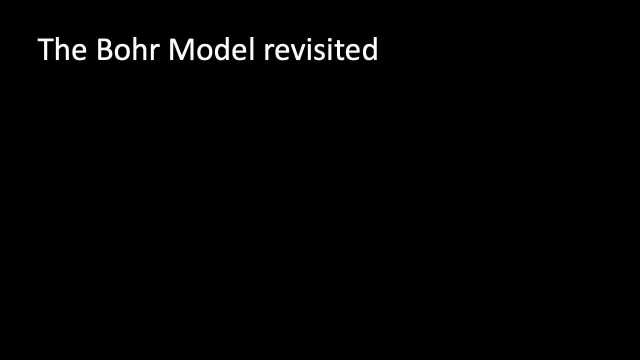 discrete energy states or orbits surrounding the nucleus. Bohr's original calculation was based on the quantization of angular momentum. If you're not familiar with this calculation, I've made a video explaining it. If you're not familiar with this calculation, I've made a video explaining it. 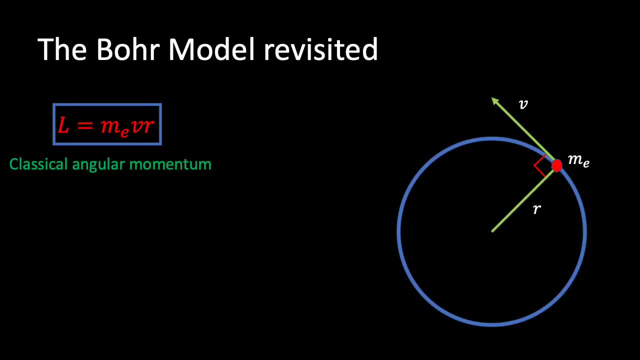 Bohr assumed that the angular momentum of the orbiting electron, which is classically given by the expression l, equals m times v times r, where v is the velocity, r is the radius and m is the mass, can only take certain values equal to an integer multiple of Planck's constant divided by 2 pi. 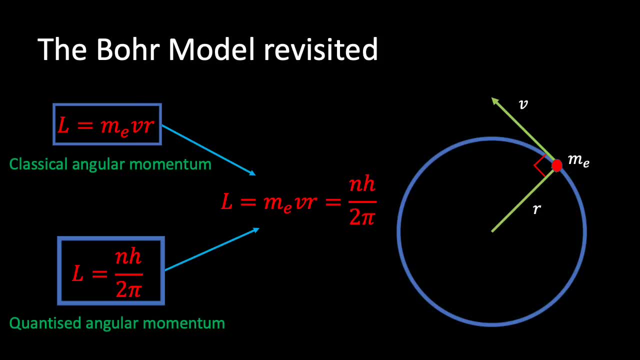 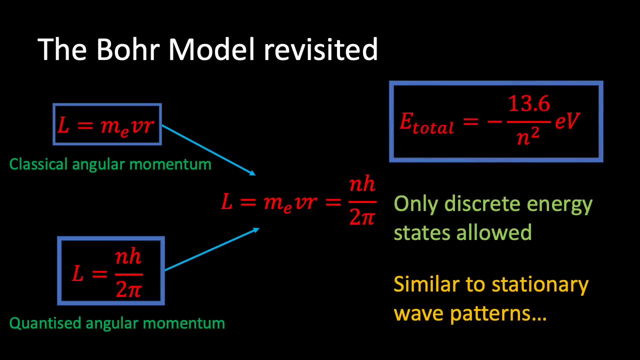 He then showed that this angular momentum condition leads to the quantization of the electron's energy and only discrete values are allowed. Specifically, the angular momentum is equal to minus 13.6 electron volts divided by n squared, where n is an integer, And recall that it was this integer restriction that reminded de Broglie of the stationary wave. 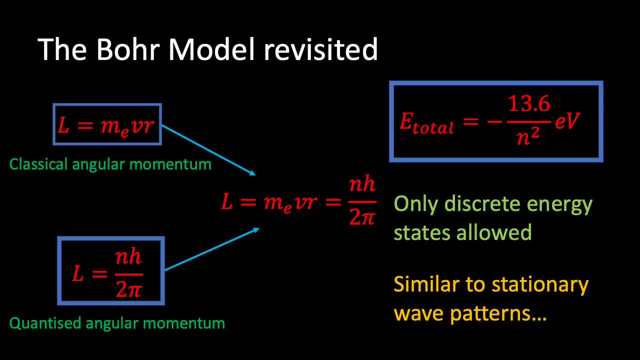 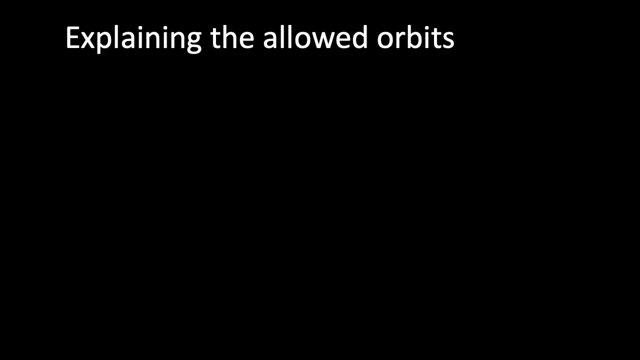 patterns created by the interference of progressive waves on strings. de Broglie proposed this whole number condition restricted the possible electron orbits in the Bohr atom to those with the circumference that permitted the formation of electron standing waves. These electron standing waves were the ones that were the most likely to form electrons standing waves. 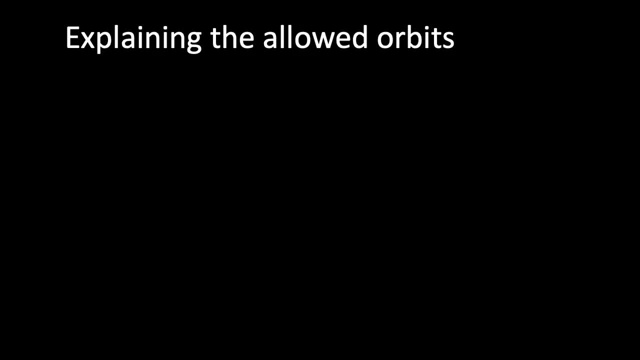 These electron standing waves were not bound at either end, like those on a musical instrument, but were formed because a whole number of wavelengths could be fitted into the circumference of the orbit. To see this, consider the angular momentum quantization condition. Recall that mv is simply the linear momentum p of the electron. Therefore we can write: pr equals. 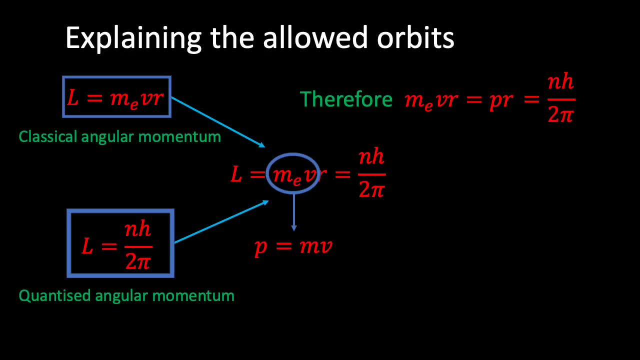 nh over 2 pi. We can then use the expression for the de Broglie wavelength p equals h over lambda to write hr equals h over lambda. If we rearrange this expression, then we see that 2 pi r equals n lambda, where n is an integer. 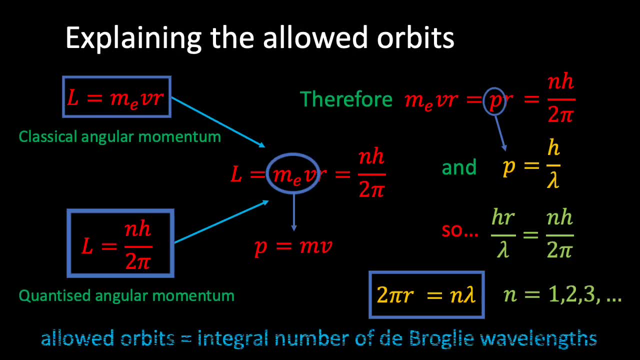 So what is this telling us? This expression is saying that the allowed orbits in the Bohr atom are precisely those orbits that have a circumference equal to an integer number of de Broglie wavelengths, and that these stationary orbits can be thought of as corresponding to stationary wave patterns. 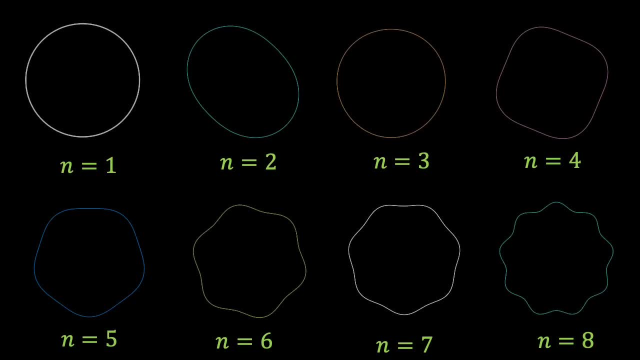 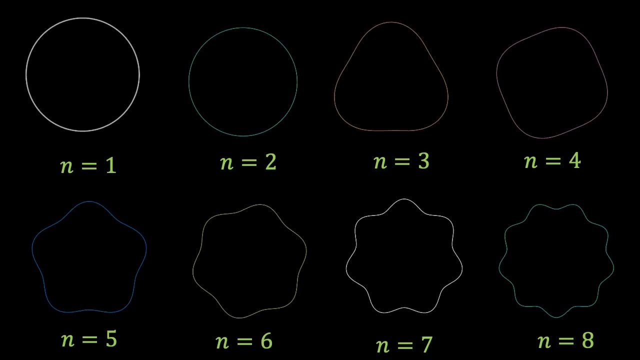 of the associated de Broglie wave. We can visualize the electron stationary wave patterns in two dimensions as follows. Note that if the distance around the nucleus is not equal to an integer number of wavelengths, then there can be no stationary wave and therefore no stationary orbit. 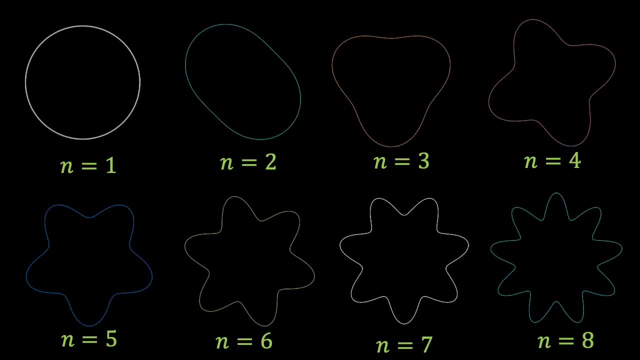 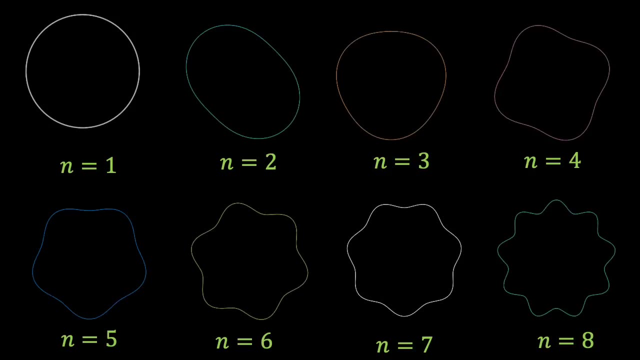 Furthermore, when viewed as a stationary wave around the nucleus, instead of a particle in orbit, an electron would experience no acceleration and therefore no continual loss of radiation, sending it crashing into the nucleus, as had been predicted by classical electromagnetic theory. What Niels Bohr had introduced simply to save his atom from collapse. 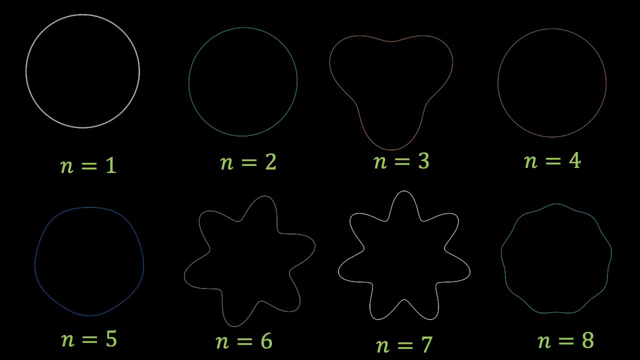 found its justification in de Broglie's wave-particle duality. De Broglie wrote up his ideas in expanded form and presented them as his PhD thesis in the spring of 1924.. One of de Broglie's four PhD examiners was eminent physicist. 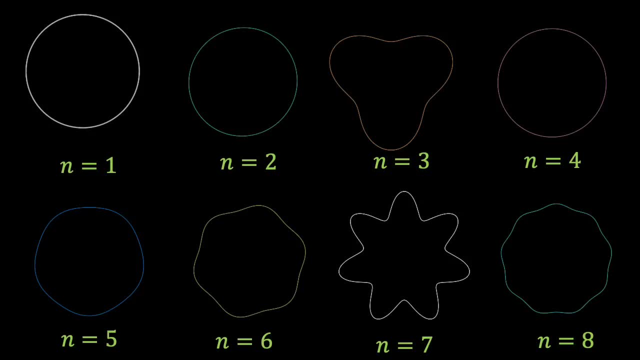 Paul Langevin. Although Langevin initially thought that de Broglie's ideas looked fancy, he didn't dismiss them, but rather sent a copy of the thesis to Einstein, who famously replied: he has lifted a corner of the great veil. Although de Broglie's ideas were theoretically enticing and had garnered the support of Einstein, 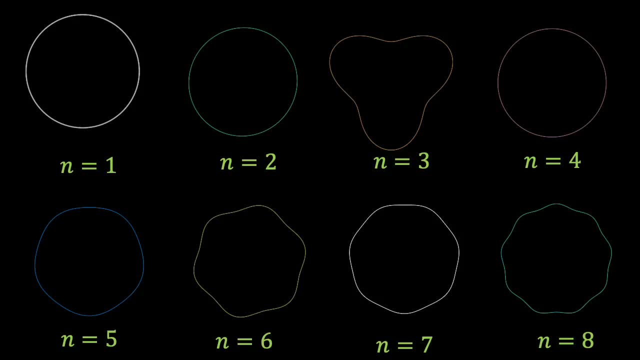 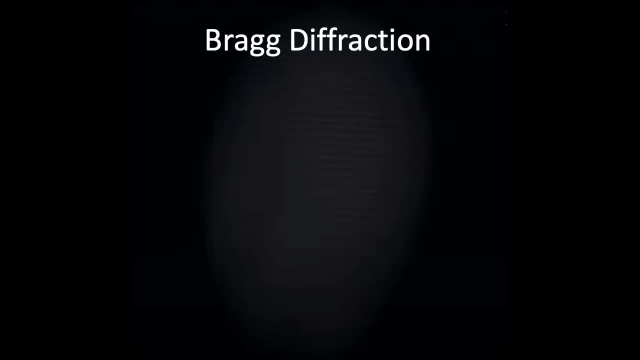 what was now needed was some form of experimental verification of the matter: wave hypothesis. One of the most exciting features of de Broglie's work was the realization that if electrons exhibited wave-like properties, then it should be possible for electrons to undergo diffraction, and 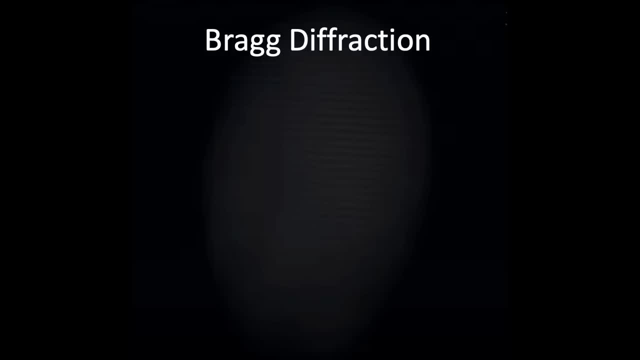 interference, just like waves do. For this to occur, the electrons would have to pass through an incredibly small gap, and the associated de Broglie wavelength of the electrons would need to be comparable to the size of the gap through which they passed. Where could you find such a? 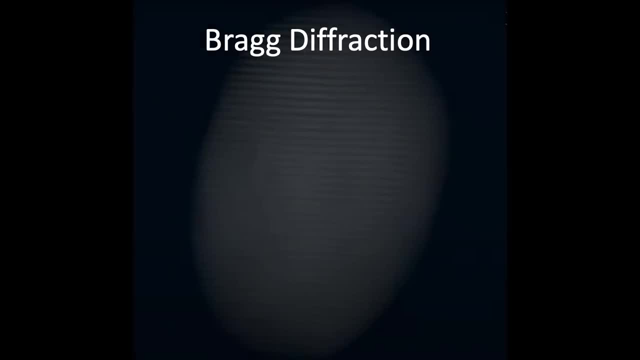 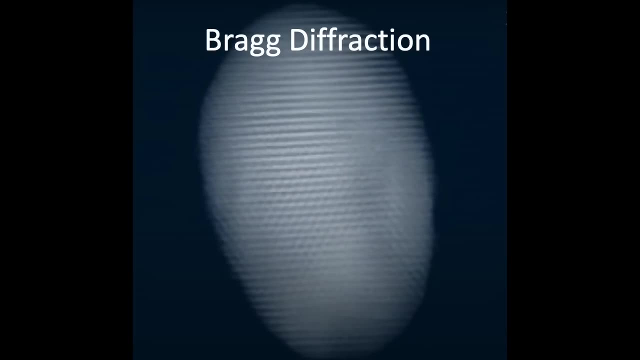 small gap. Fortunately, nature had already provided the answer in the form of crystal lattices. A crystal lattice consists of a reddish glow and is winch shaped of a regularly spaced array of ions, with a suitably small gap separating each plane. 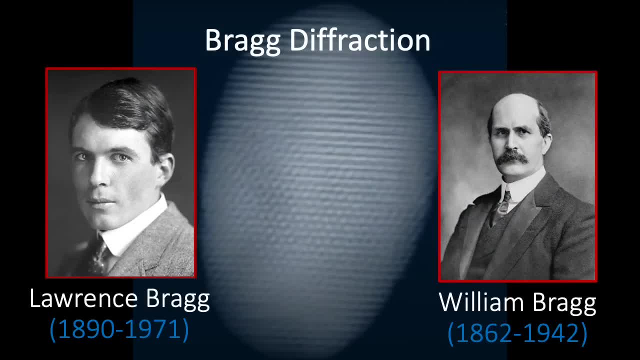 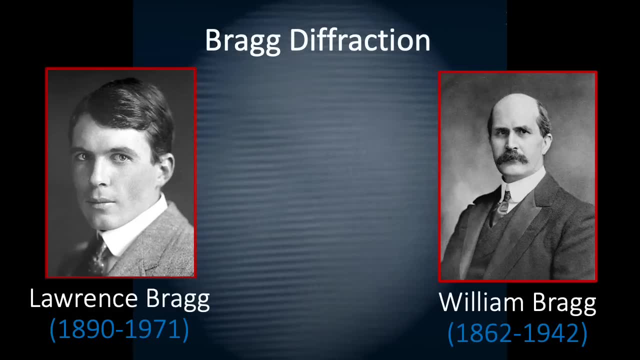 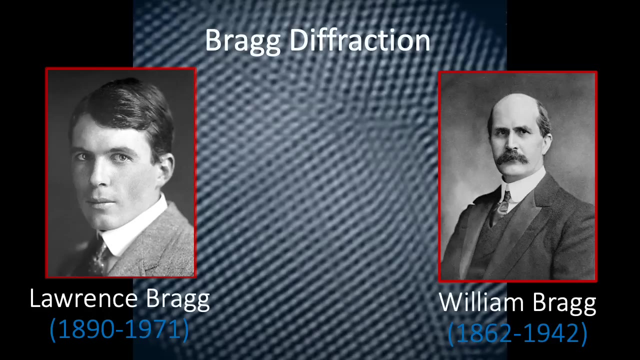 In 1914, William Bragg and his son, Lawrence Bragg, demonstrated that it was possible to scatter x-rays using a crystalline solid. They found sharp peaks in intensity at certain x-ray scattering angles, which they interpreted as diffraction maxima. They were able to use the x-ray diffraction 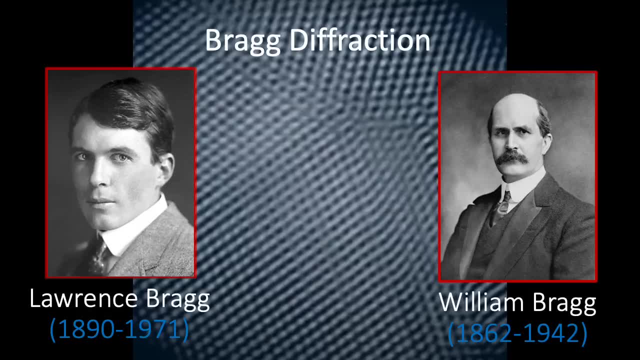 patterns to reconstruct the crystal structures of the solids that they were investigating. Now, if this is true for x-rays, then perhaps a similar phenomena can be observed for electrons. if they do, as de Broglie had suggested, have wave-like properties, The atoms of this solid 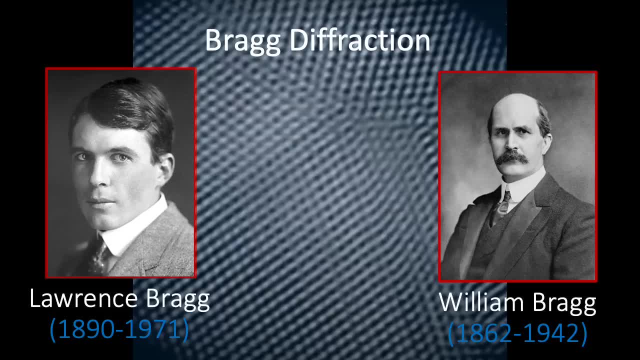 act as a three-dimensional array of diffracting centres for the electron matter waves, meaning that, much like with x-ray diffraction, electrons should be scattered in certain characteristic directions. This idea was confirmed in a series of experiments conducted by Clinton Davison and. 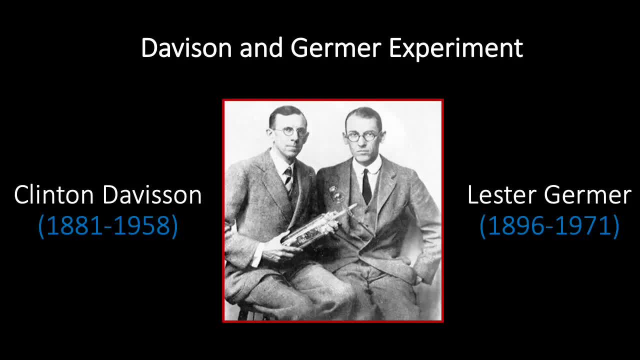 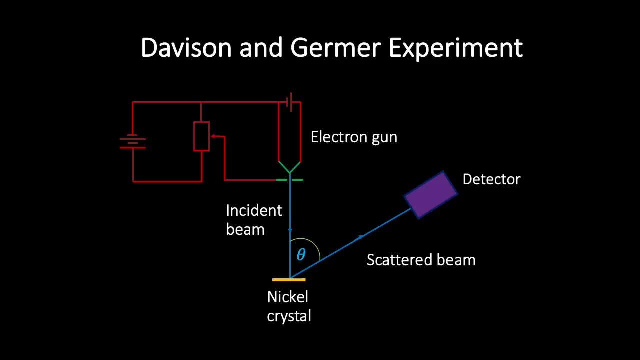 Lester Germer in the 19th century. The idea was that the x-ray diffraction of electrons in the United States between 1923 and 1927. The experiments involved accelerating electrons through a particular voltage and then scattering them off a regular crystalline solid. similar. 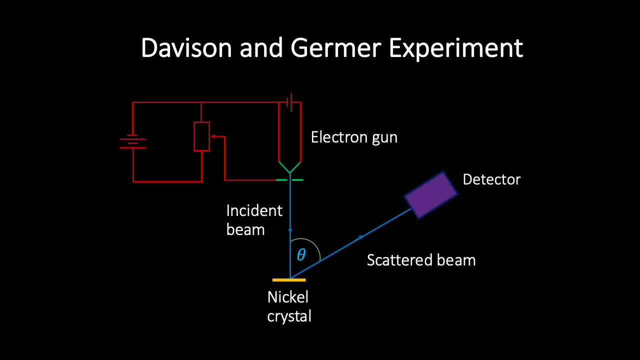 to the scattering experiment conducted by Bragg with x-rays. The detector is set at a particular angle, theta and readings of the intensity of the scattered beam are taken at various values of the accelerating potential. The accelerating potential can be used to change the speed and therefore the de Broglie wavelength, of the electrons inside the beam. 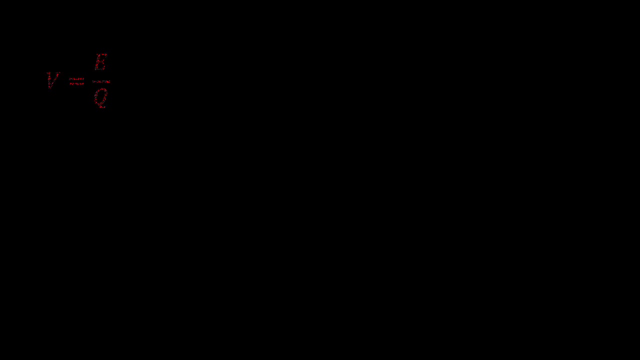 To see this, recall that potential difference or voltage is defined as the energy transferred per unit charge. Therefore, the energy transferred to a single electron passing through a potential difference V is given by E equals eV, where little e is the charge of the electron, 1.6. 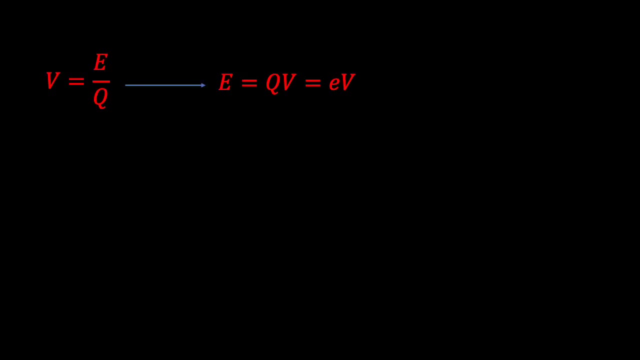 times 10 to the minus 19 coulombs. This energy is transferred into the kinetic energy of the electron, and so we can write: eV equals half mv squared, And so we see that the speed of the electron in the beam is given by the square root of 2eV over m, And therefore the de Broglie. 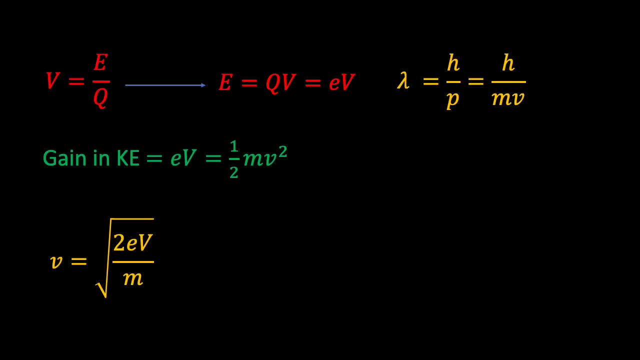 wavelength, which is written as lambda, equals h over p. which is equal to h over mv, can be written as h divided by the square root of 2m eV. So we see explicitly how the variation of the accelerating potential difference can be written as the speed of the electron in. 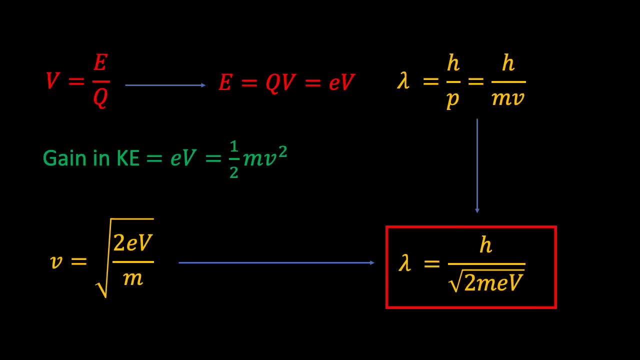 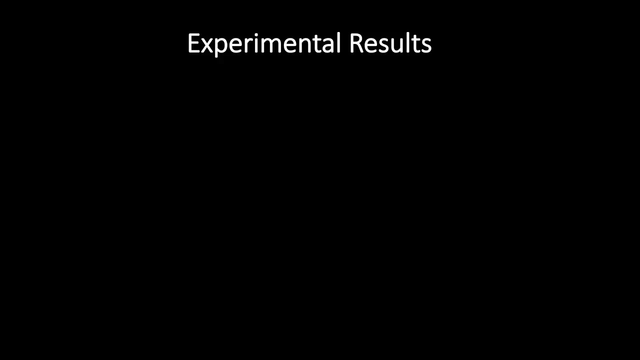 a ray called the de defined leastleigh, which is a Otringte of not that large of an angle. bu f e m f N p rays. m r s was e company at an electron energy of 54 electron volts If an appreciably smaller or larger angle than 50. 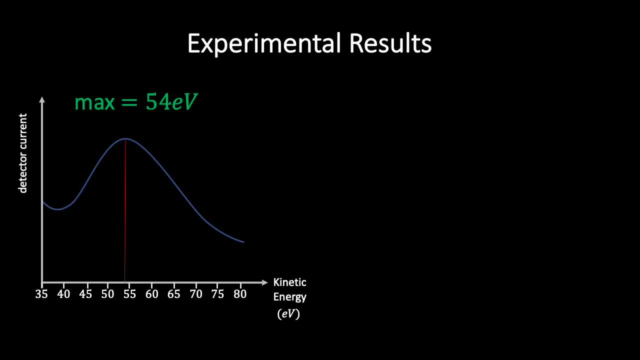 degrees is used, the diffraction maximum disappears. This can be seen by plotting a graph of detector current as a function of detector angle for the fixed value of electron kinetic energy of 54 electron volts. The existence of this peak in the electron scattering pattern. 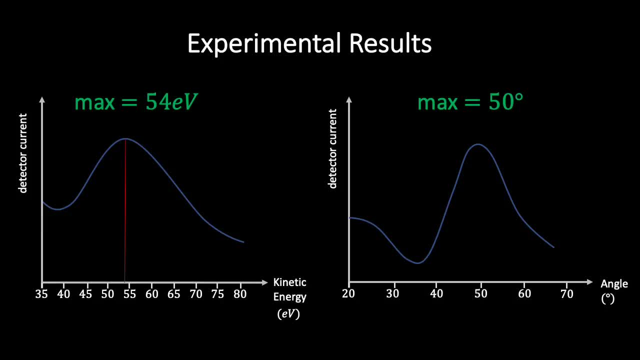 demonstrates qualitatively the validity of de Broglie's postulate, because it can only be explained as a constructive interference of waves scattered by the periodic arrangement of the atoms into planes of the crystal. The phenomenon is precisely analogous to the well-known Bragg 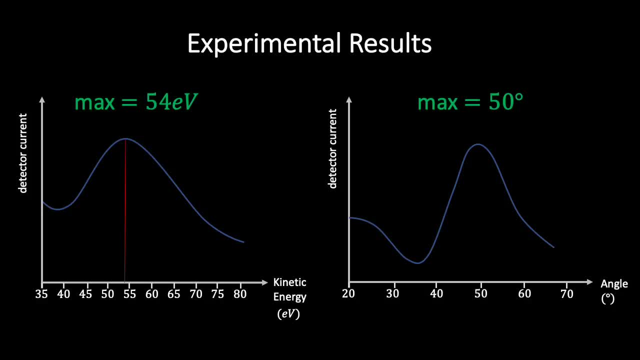 reflections which occur in the scattering of x-rays from the atomic planes of a crystal. It cannot be understood on the basis of classical particle motion, but only on the basis of wave motion. Classical particles cannot exhibit interference, but waves can. The interference involved here is not between waves associated with one another. 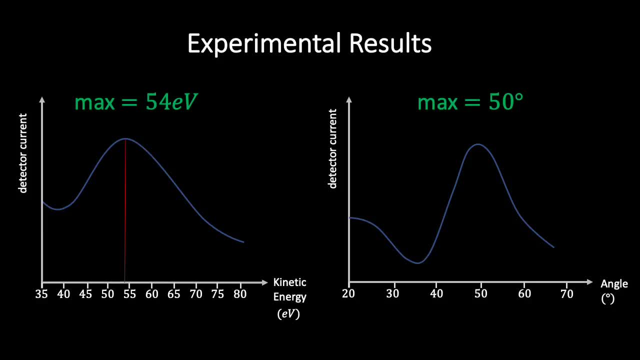 Instead, it is an interference between different parts of the wave associated with the single electron that have been scattered from various regions of the crystal. This can be demonstrated by using an electron beam of such low intensity that the electrons go through the apparatus one at a time, and by showing that the pattern of the scattered electrons remains the same. 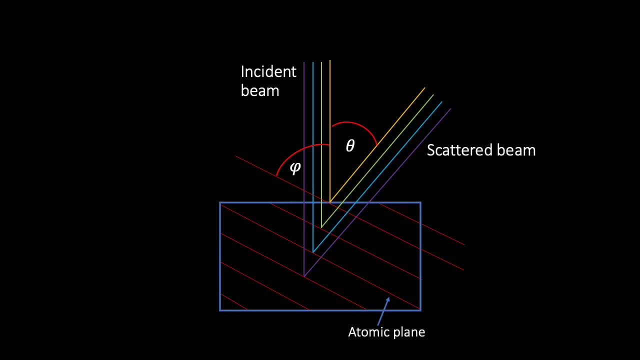 The strong diffracted beam at theta equals 50 degrees and 54 electron volts. over the electron beam is. a strong diffracted beam at theta equals 50 degrees and 54 electron volts. It arises from the wave-like scattering from the family of atomic planes. 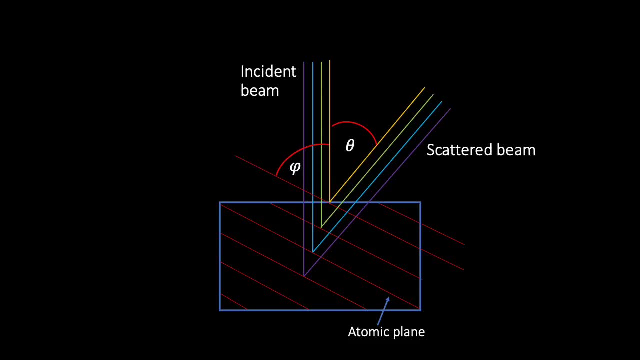 which can be seen in the diagram. The techniques of x-ray diffraction had already been used to show that these atomic planes had a separation of roughly 9.1 times 10 to the minus 11 meters. Furthermore, as we have already seen, Davison and Germer's experiment had shown that the scattering 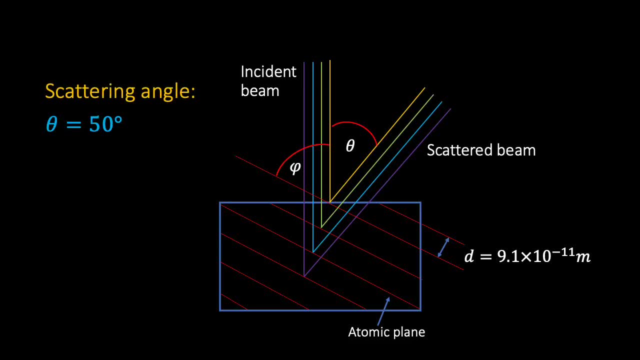 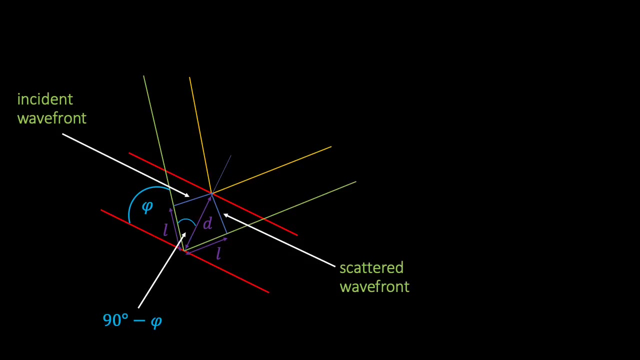 angle corresponding to maximum diffraction was at 50 degrees and therefore the angle phi, known as the Bragg angle, was 65. degrees. If we next focus in on just two of the atomic planes and two rays of the incident and scattered beams, then we see that when an integral number of wavelengths n lambda fits into the 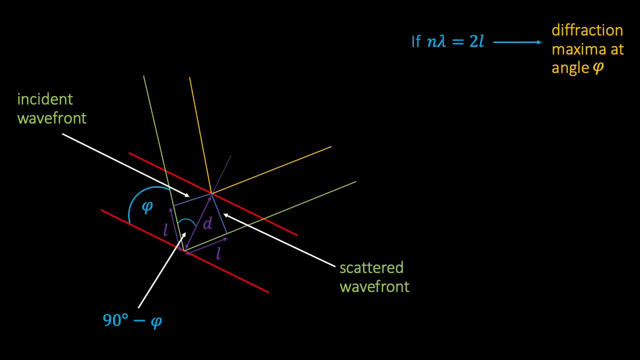 distance 2l, then the contributions along the two rays to the scattered wavefront will be in phase and a diffraction maximum will be attained at an angle phi. Now, since l over d equals cos 90 minus phi, and since this is equal to sine of phi, we then have that 2l equals 2d sine phi, and therefore 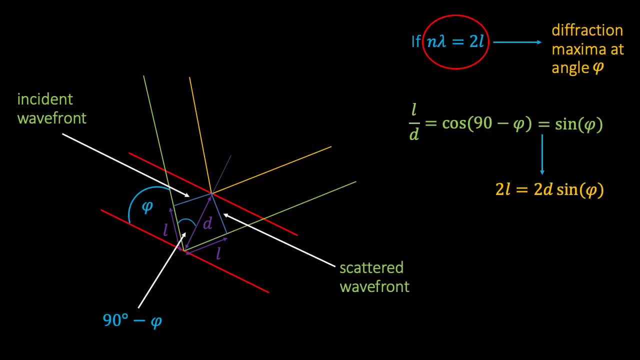 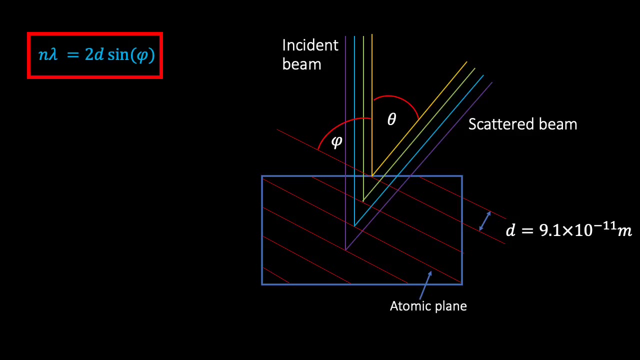 if we use the relationship n lambda equals 2l and combine this with the relationship 2l equals 2d sine phi, we finally arrive at the Bragg relation n lambda equals 2d sine phi. Now the first order: diffraction maximum corresponding to n equals 1 is usually the most. 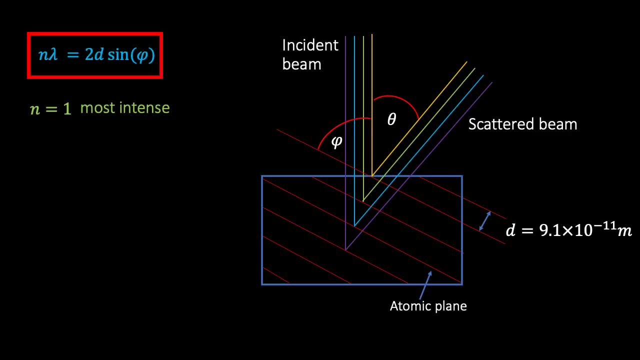 intense, and for the particular case that we've been considering, the Bragg angle phi is equal to 65 degrees, and so lambda is given by 2d sine 65. We also know that d equals 9.1 times 10 to the minus. 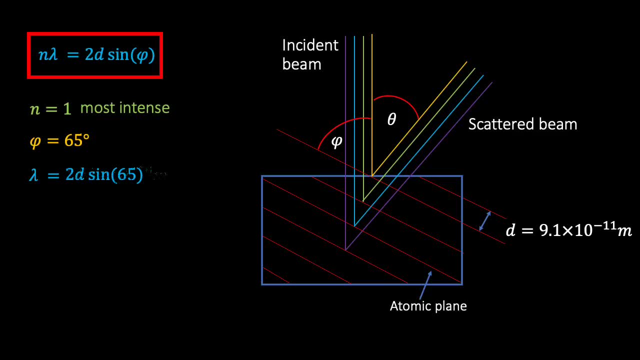 11 meters and therefore we find from the Bragg equation that lambda equals 1.65 times 10 to the minus 10 meters. We can then compare this wavelength with the de Broglie wavelength of an electron with the Bragg value. Recall that the de Broglie wavelength can be calculated using the following equation: 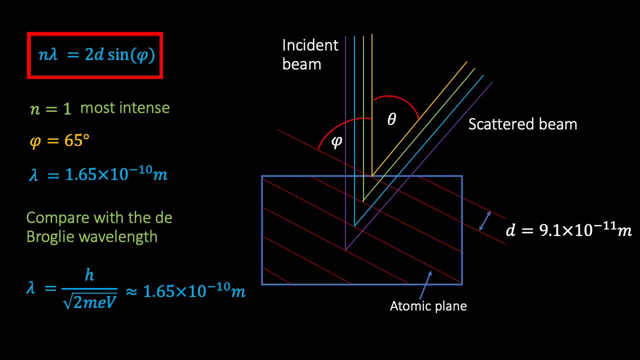 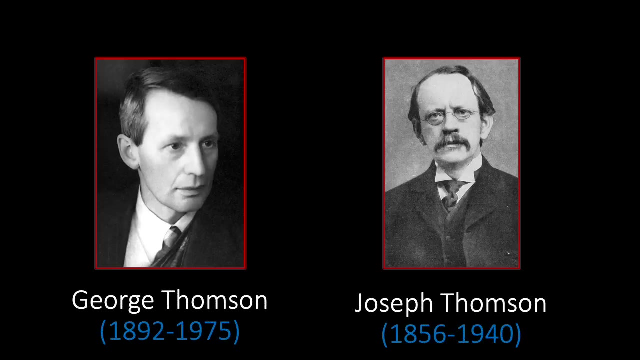 and if we put in the numbers we find remarkable agreement with the Bragg value. This impressive agreement between theory and experiment provides quantitative confirmation of the de Broglie relation between lambda p and h. In 1927, George Thompson, son of JJ Thompson, independently confirmed. 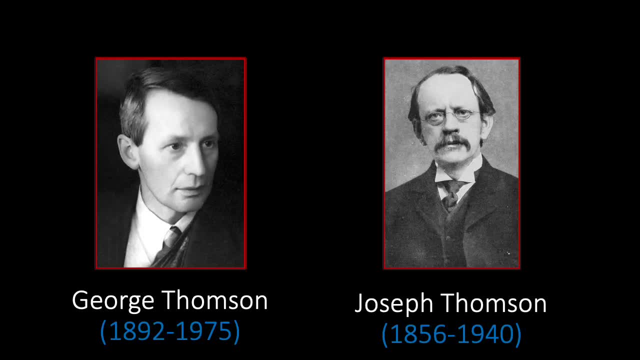 the de Broglie relation using high energy electrons. It's of interest that JJ Thompson, who in 1897 discovered the electron which he characterized as a particle and for which he was awarded the Nobel Prize in 1906, was the father of George Thompson. 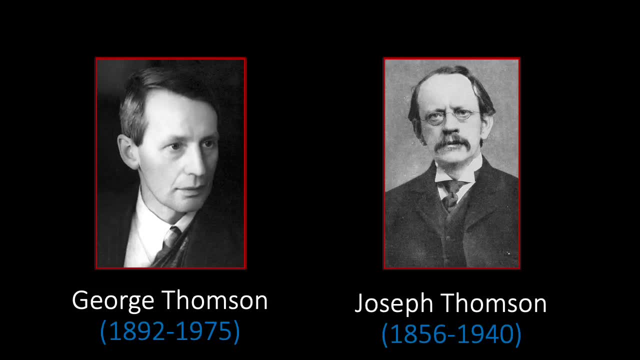 who in 1927 experimentally discovered electron diffraction and was awarded the Nobel Prize with Davison in 1937. Max Jammer writes of this. one may feel inclined to say that Thompson, the father, was awarded the Nobel Prize for having shown that the electron is a particle. 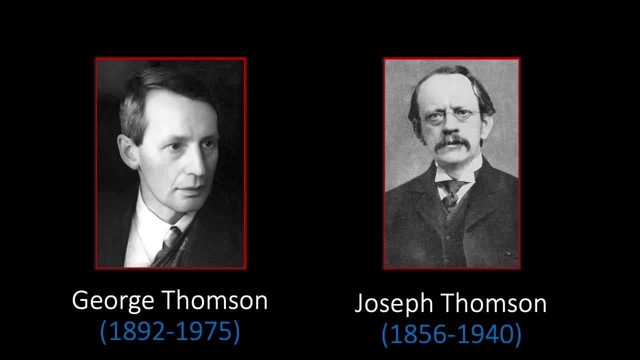 and Thompson, the son, for having shown that the electron is a wave, But this would be oversimplifying the situation. Although the experiments of Davison, Germer and Thompson had demonstrated the wave-like behaviour of the electron, there was still a great deal. 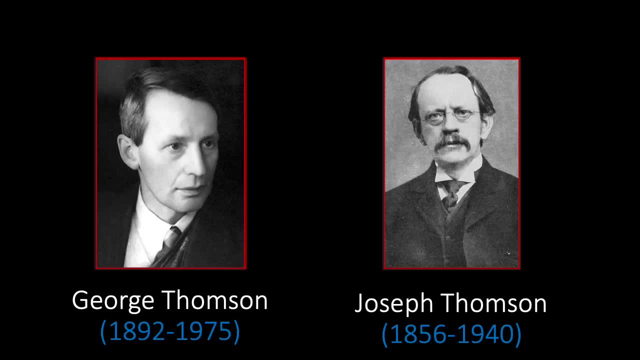 of uncertainty surrounding the physical interpretation of the results. What does it mean to say that the electron behaves like a wave? Does this mean that the electron is a wave? And when we assign a de Broglie wavelength to a material particle, what does this wavelength represent? 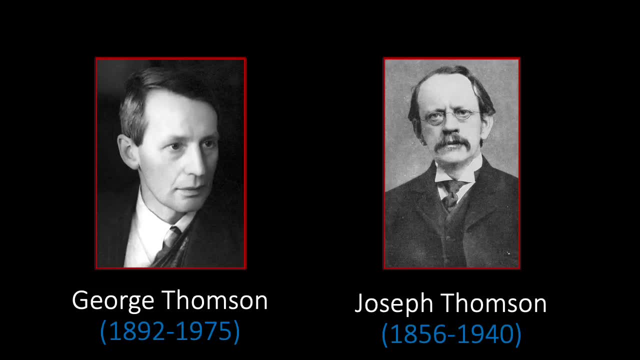 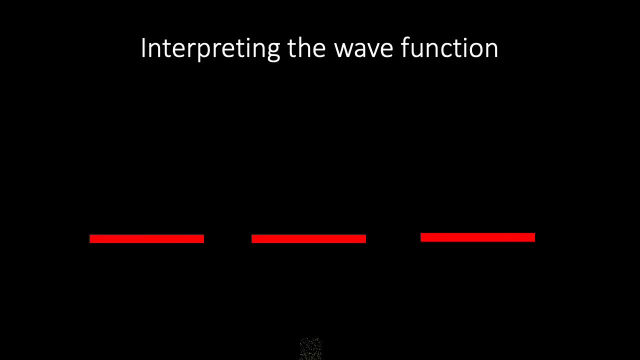 Does it represent the length of a real wave Or is it something more abstract? To answer this question, we will return to one of the most famous experiments in physics: the double slit experiment. We will begin by considering a classical physics setup in which we imagine firing a stream of 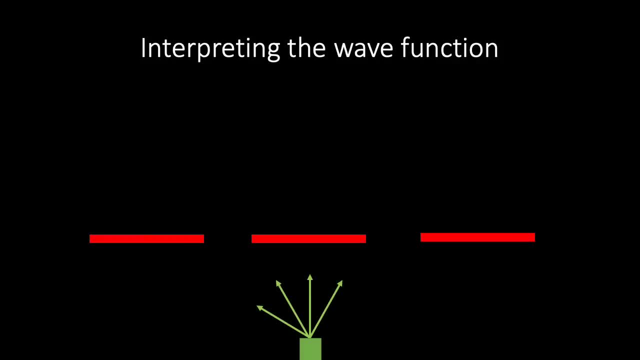 indestructible tennis balls at an indestructible sheet of metal which contains two parallel slits. On the other side of the parallel slits is a detector consisting of a bucket that can be moved along an axis. Imagine that in a certain amount of time, on average, a thousand tennis 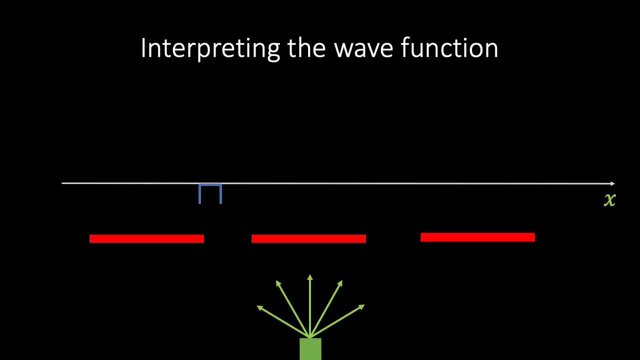 balls are fired towards the two slits. Next, consider moving the detector along the x-axis and, for each location, counting how many balls are collected in the bucket during the set amount of time. In other words, count how many of the 1,000 balls fired end up in the 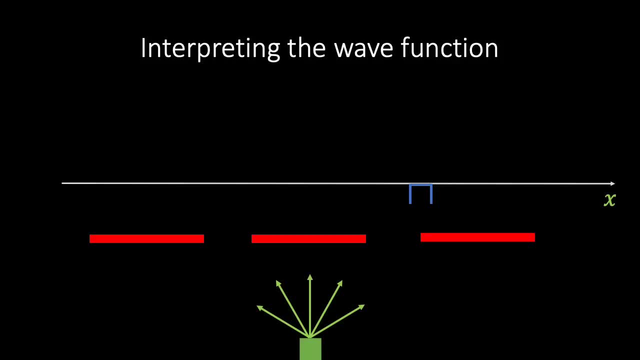 bucket at each x-location. You can see that counting the number of balls at each location will tell you the probability that the detector will move along an axis. In this example, we can see the probability of finding a ball at a particular location in a certain period of time. 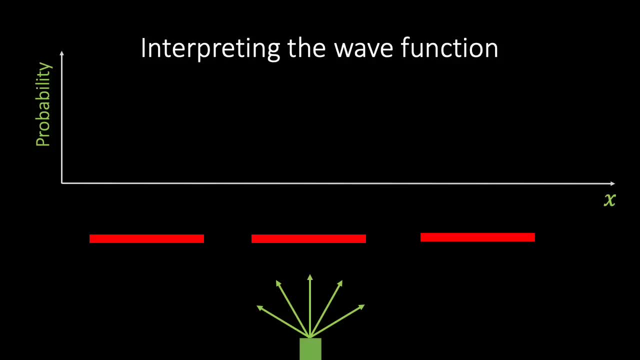 We could repeat this experiment very many times and plot the probability distribution. It is clear that we would expect the probability distribution to peak around the two slits, And indeed this is what we find. Next, let us consider a similar experiment. only this time we will send. 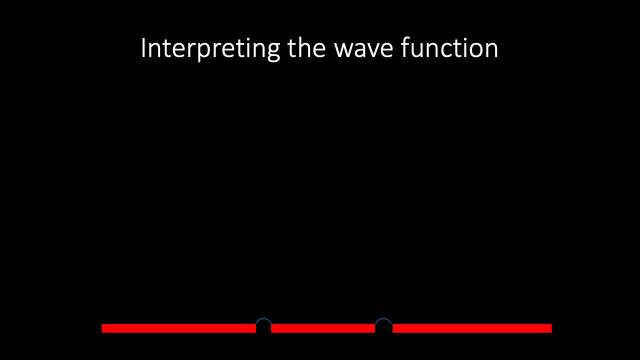 water waves towards the two slits, rather than tennis balls. Water waves are different from balls in the field of a ball. In this example, the water waves are different from balls in the that they spread out over space and are subject to the principle of superposition, which we 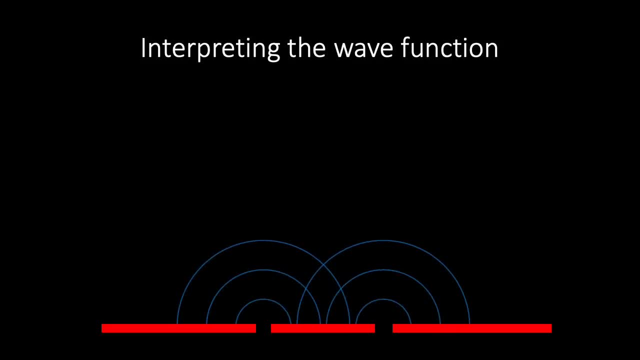 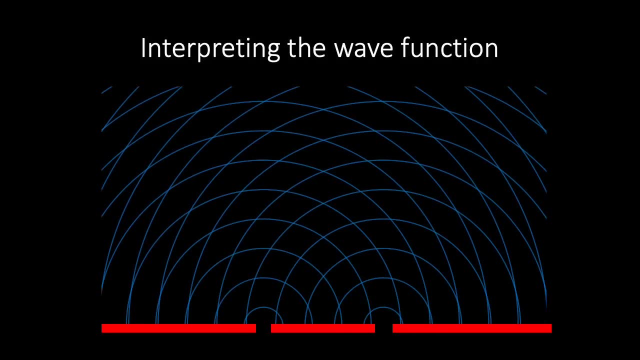 encountered earlier. As the waves pass through the two slits, diffraction will occur at each slit, causing two sets of overlapping waves. Recall that the principle of superposition states that the net displacement of the water at any point in space will be equal to the sum. 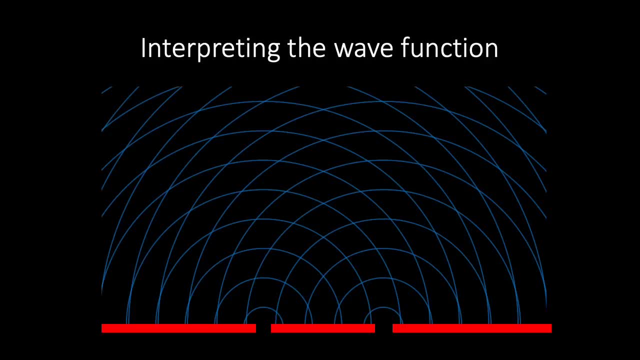 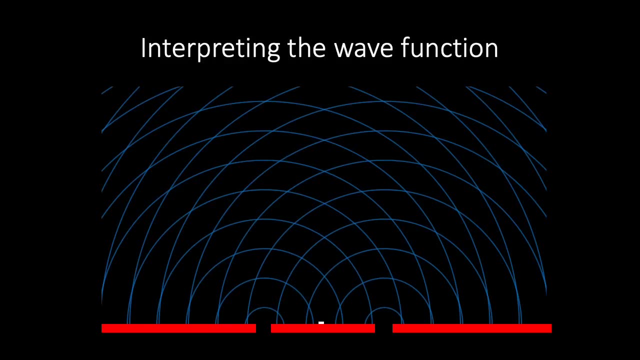 of the individual displacements of each wave passing through that point at a particular moment in time and therefore there will be locations in which the water waves reinforce one another, producing a large net displacement, and there will be locations where the water waves cancel each other, producing a net displacement of zero. On the other side of the slits, we will 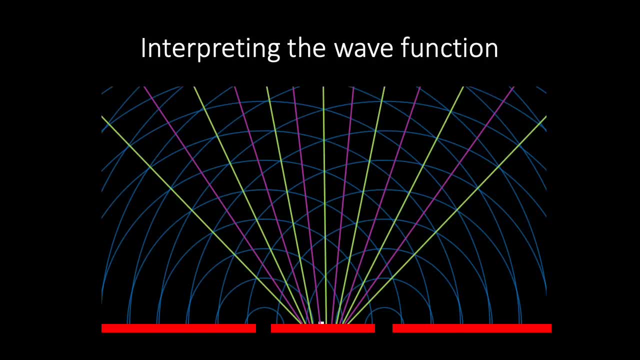 have a detector that records the intensity of the wave. Now, the intensity of a wave is proportional to the energy carried by the wave, and the energy carried by the wave is proportional to the square of the amplitude of the wave. So, for example, our intensity detector might consist of a bob that floats in the water and by recording 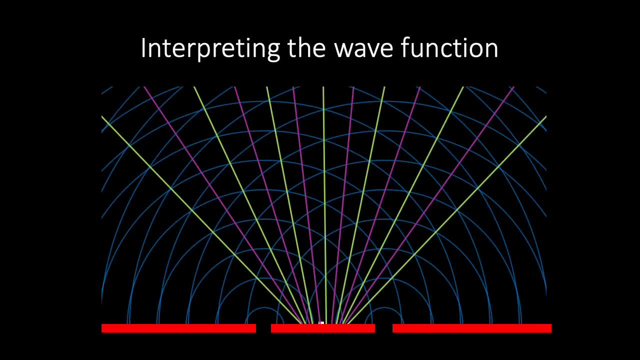 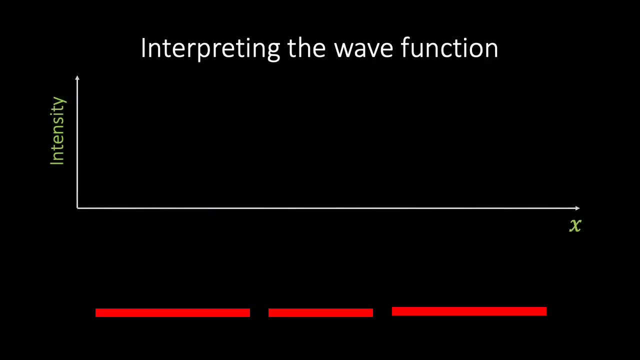 the maximum displacement or amplitude of the bob, we would be able to calculate the intensity of the wave. If we then plot a graph with intensity on the y-axis and position on the x-axis, then we would find the following result: The shape of the graph reflects the fact that 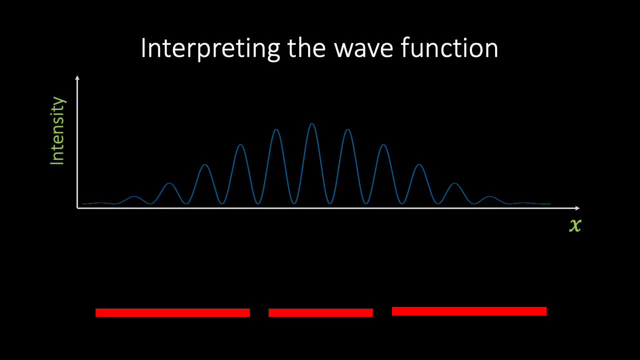 there are certain regions where the waves reinforce one another and certain regions where the waves cancel. And just to emphasise, the intensity at any location is proportional to the square of the wave amplitude at that point. Next, let us consider performing the same experiment, only this time we will fire electrons. 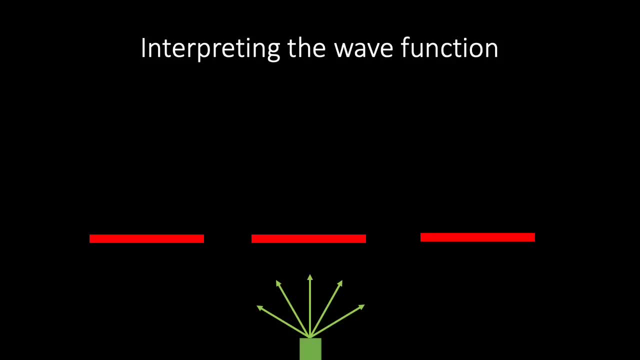 at the parallel slits. A few things are important to emphasise. When our detector detects an electron, it only ever detects a whole electron or no electron. It never detects a fraction of an electron. In other words, our electrons are indestructible fundamental units. Secondly, 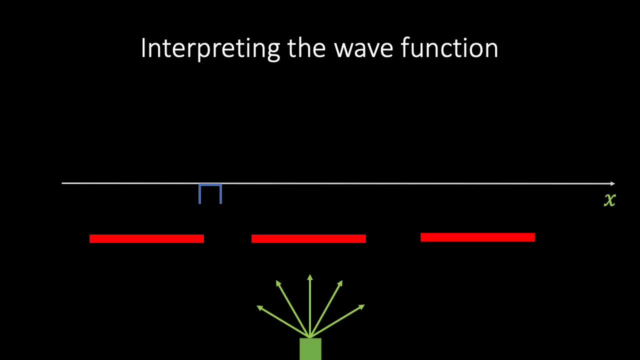 it is never the case that the electrons are indestructible units. It is never the case that when electrons are fired at the slits one by one, two detections can occur simultaneously. These detections always occur at a single spatial location. We see that this situation 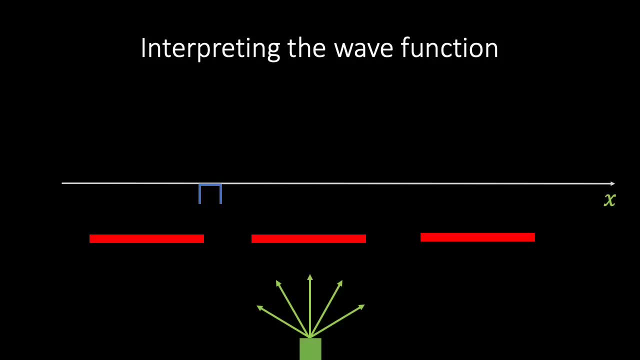 is very much, very similar to our original tennis ball experiment, only that we have replaced tennis balls with electrons and buckets with electron detectors. Just like with the tennis ball example, we can calculate the probability that an electron will end up at a certain x location in a given amount of time. What results do we expect? 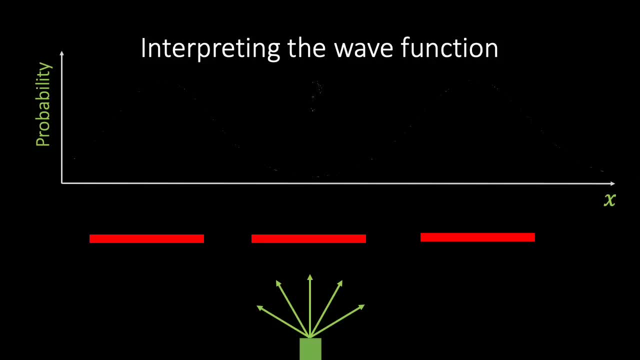 Surely it's the same as for the tennis balls, right? We should expect two peaks corresponding to the two slits. Well, this is not what we get when we perform the experiment. When we actually perform this experiment with electrons, we find the following remarkable result: 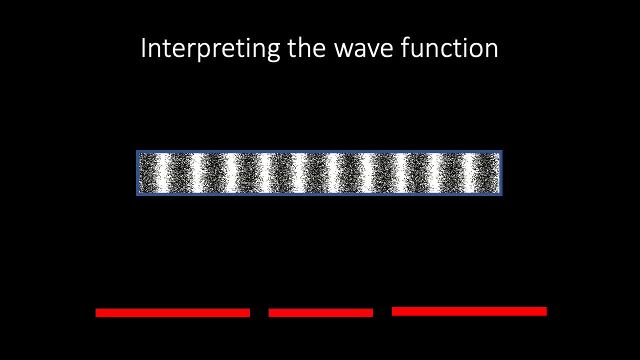 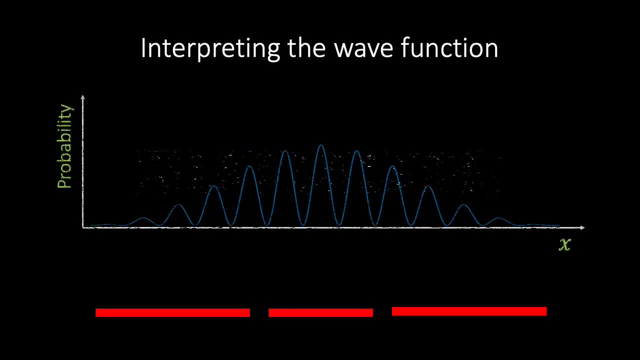 We see clearly that there are alternating regions where the electrons can and can't be detected, similar to the light and dark fringes observed by Thomas Young all those years ago. If we plot the corresponding probability curve, then we find that the probability distribution corresponding to electron location 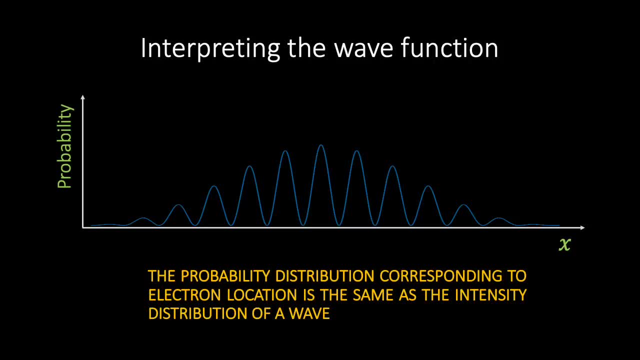 is the same as the intensity distribution of a wave, And this is the deep link that we've been looking for between so-called wave and particle pictures of reality. The wave we associate with an electron tells us something about the probability of finding the electron at a particular location in space at a particular moment in time.